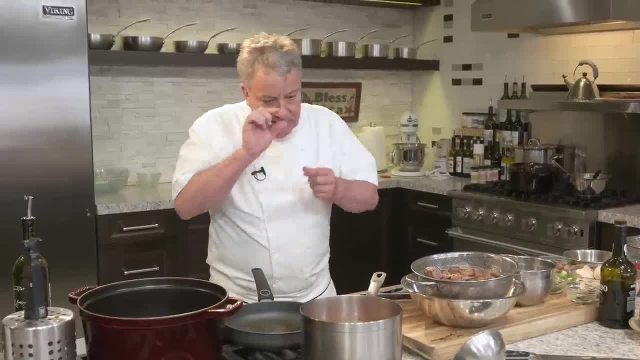 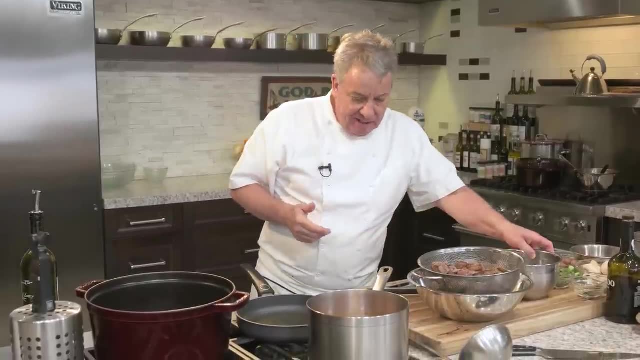 couldn't get them, Cipollini. Cipollini is a little flat onion, but that big right there it's a little flat And it's really, really delicious. but I couldn't find any, So I got the onion right there. 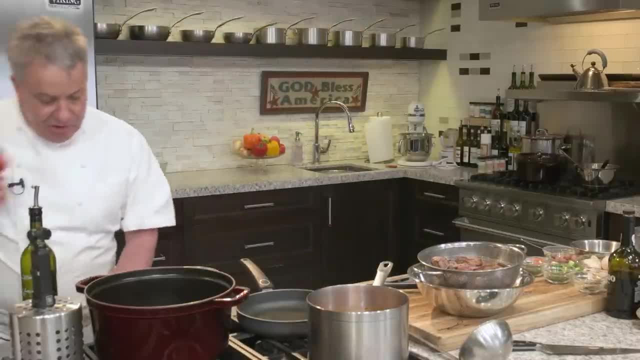 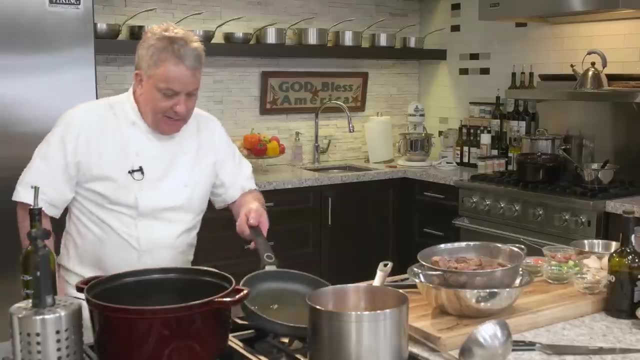 the pearl onion. I'm going to put them in my oil. Let me double check to make sure my pan is hot. I want it to be about 365, and then I'm going to saute my beef. I wanted to show you. 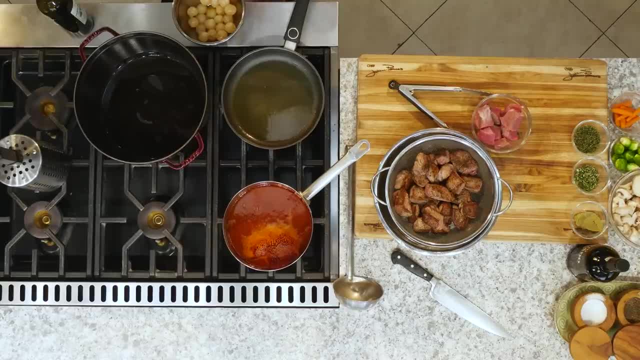 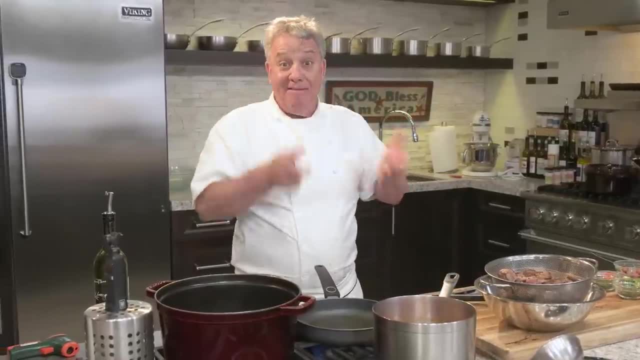 by the way, you see, I got everything ready. I got everything ready, meaning that my mise en place is ready, Everything is chopped and ready to go. I just have a few more things, and the things that I have in down is because I want to show you how to. 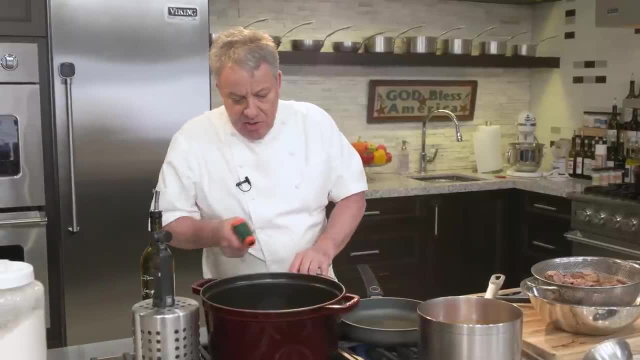 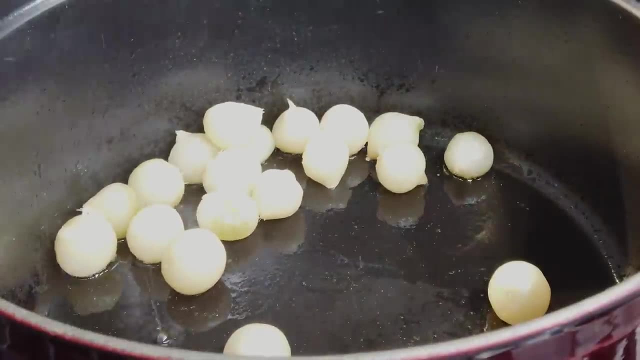 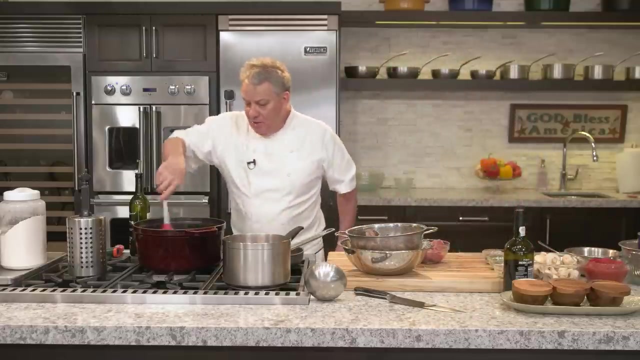 do it All right. so first we're going to saute the onion, We're going to caramelize them. The onion is always number one. always, The onion is always number one. That means it's always the first ingredient you put in. Okay, I don't care if you got a pearl onion, if you got cipollini. 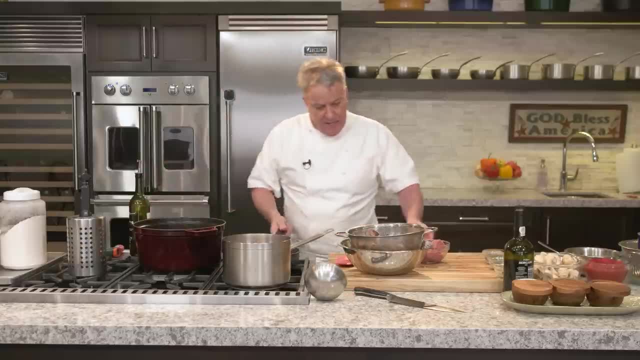 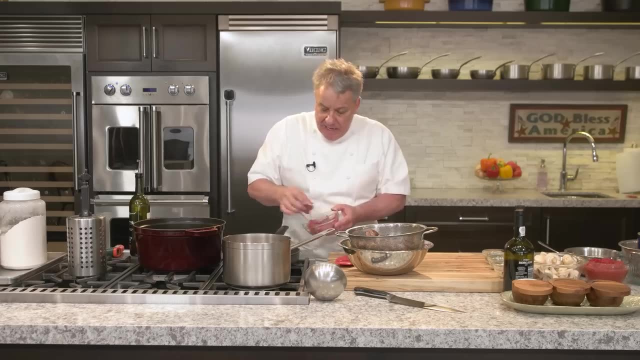 onion. if you got a red onion, you got. you want to caramelize them, right. So now this is the beef, then we're going to use this is a chuck roast. I find that chuck roast makes the beef stew. 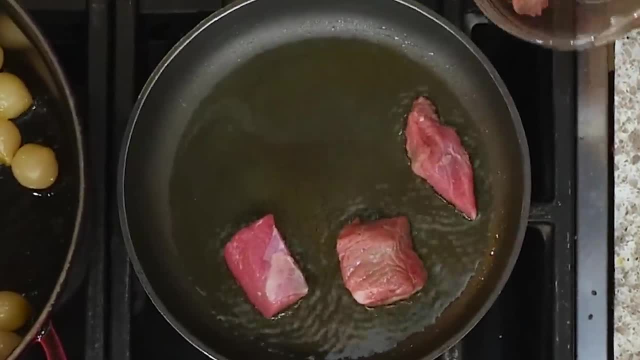 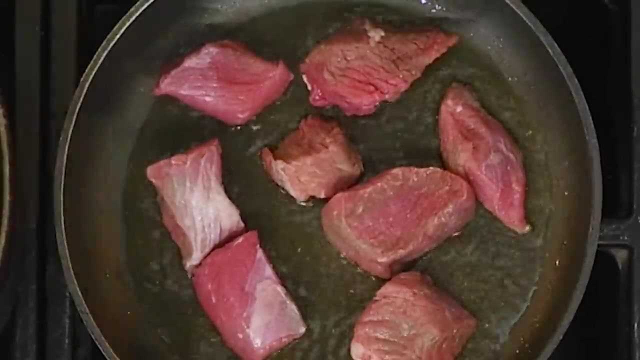 the best stew. We're going to really, really, really caramelize them so they look real pretty. okay, Not only do they look pretty, but we're creating this mala reaction where we have some caramelization of the protein. It's very important, friends, Really really important, So 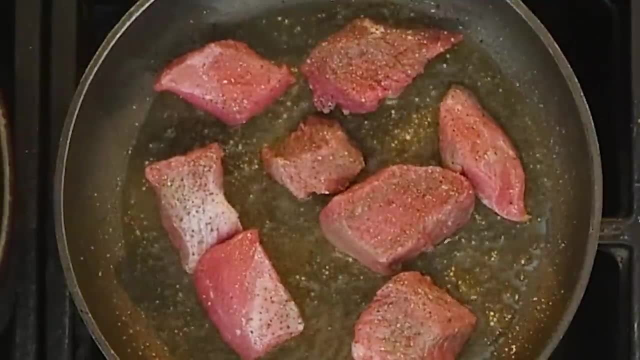 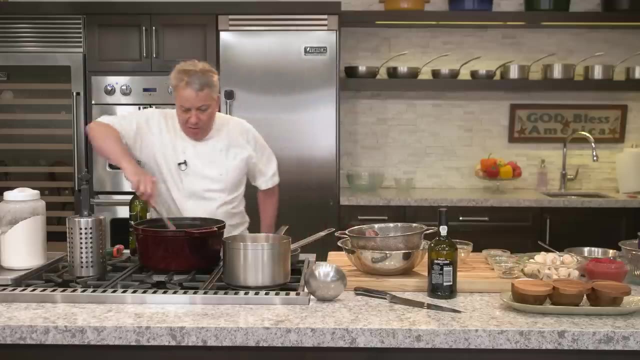 salt and pepper. Don't be afraid to put salt and pepper right, And we're going to put them in there. Don't touch them. Leave them alone. Let them get golden brown. okay, Same deal with the onion. Leave them alone. Let them do their thing. right, I got everything ready. You're going to love this. 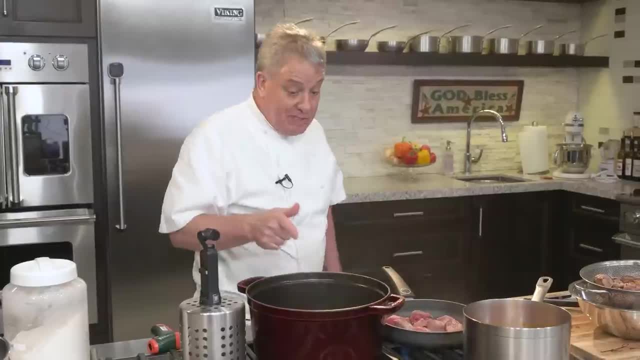 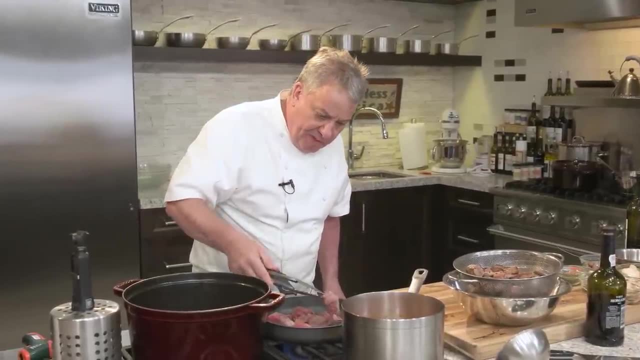 recipe It's. I got port wine in this recipe. I'm going to have port wine in this recipe. Then I got mushrooms and I got a bunch of vegetables also, but I'm going to put the vegetables toward the end. Remember, when you do this, you heard the expression. it says: 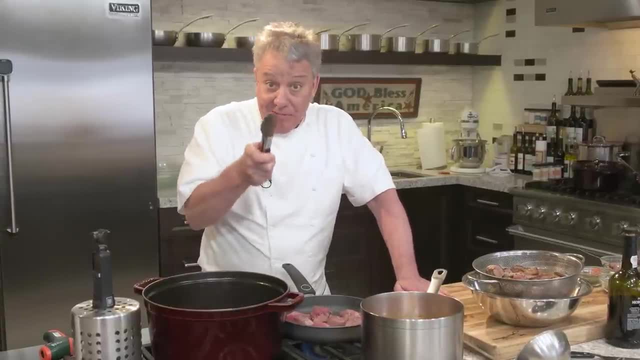 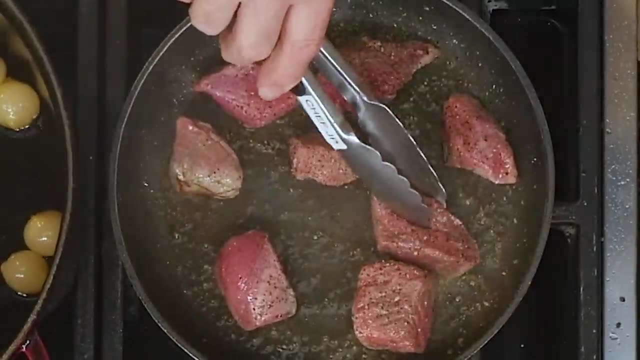 put the beef in a pan without crowding. right, Without crowding, That means don't do this, Don't put them on top of each other, Otherwise the moisture of this guy is going to go to this one is going to go to this one. 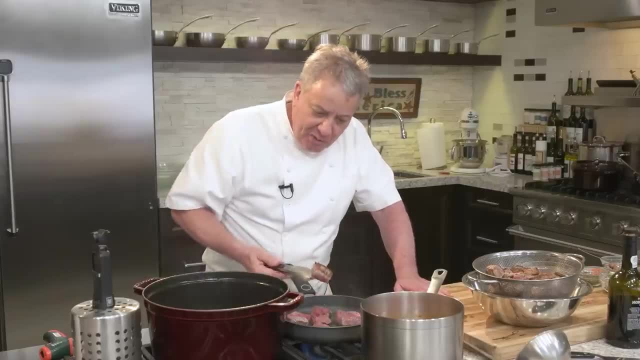 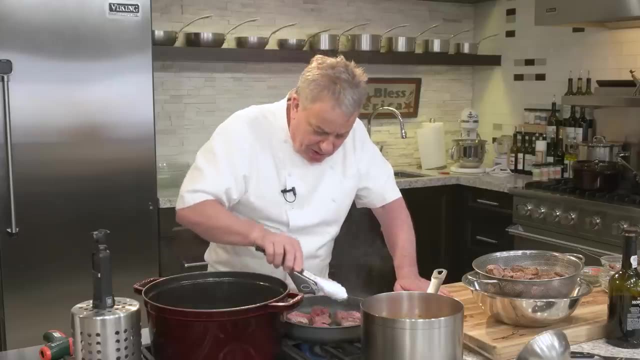 and we're going to stew, And if we stew, we don't get this caramelization right there. See it? See what I'm talking about right there? That's what I want right there, that caramelization, okay. So look, that's why you don't touch it. You put them in, leave them alone. 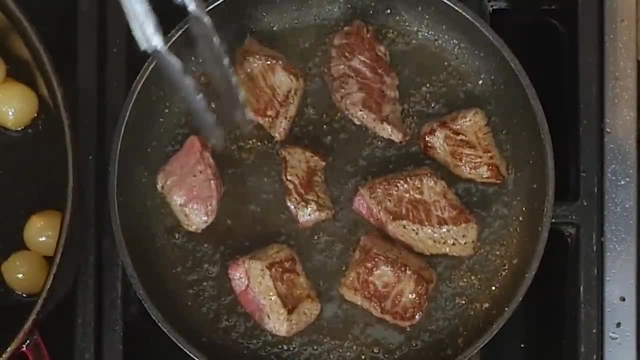 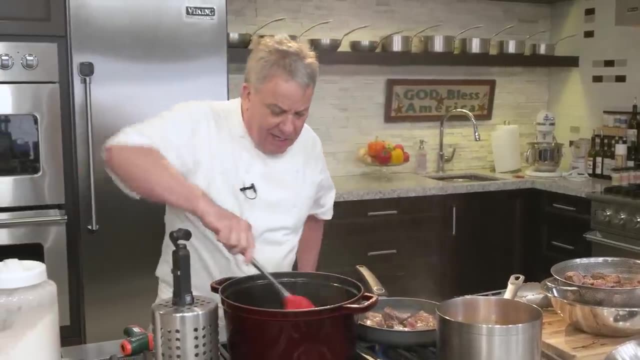 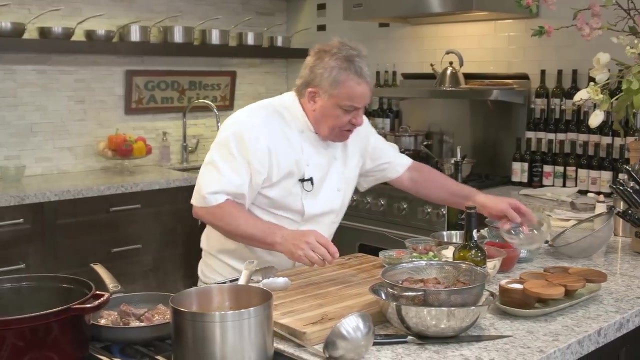 No different than if I took a New York shrimp or a filet mignon and I'm cooking it in the pan. I leave it alone. all right, I leave it alone. so it has an opportunity to caramelize. right, The onion are going to start caramelizing. The beef is right here. I got some mushrooms. 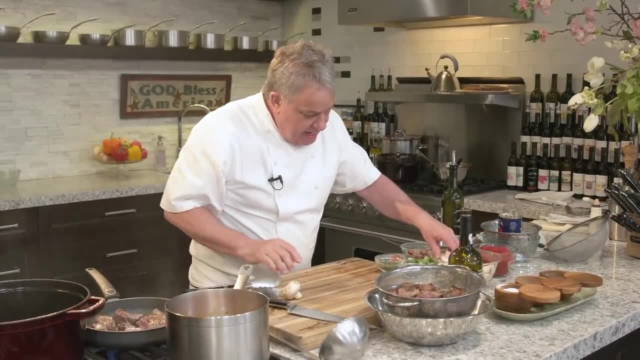 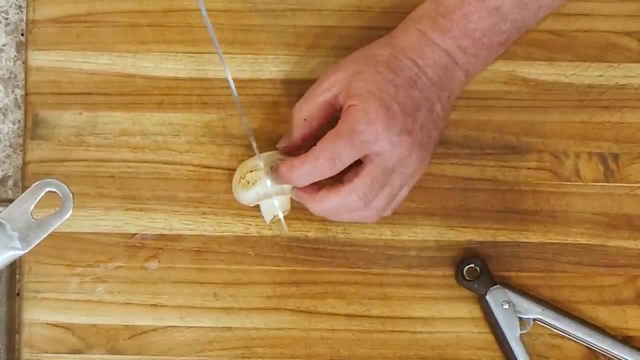 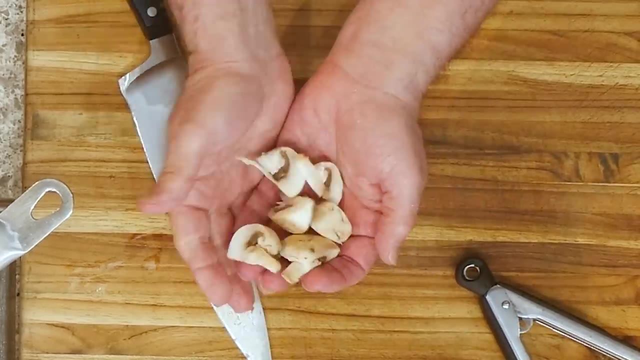 in here, friends, that we're going to use. And you know, what I like to do is, when I eat a mushroom, I do not slice them, I cut them in quarters. If they're too big, I cut them in eight or six, so they stay nice. 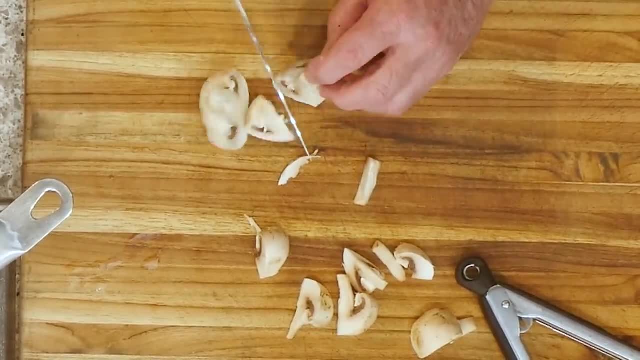 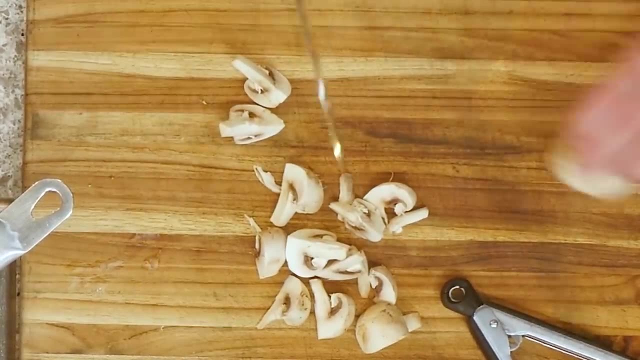 You see what I mean. You don't slice them. Like I said, if they're very big, cut them in six. okay, If they're small, just cut them in quarters. It doesn't really matter. but you don't want to slice them, okay, See, look, cut them in sixes, all right. 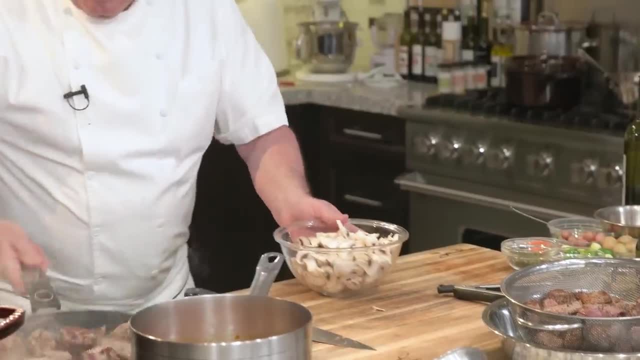 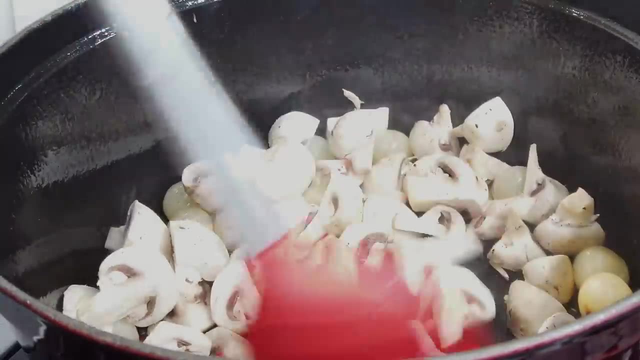 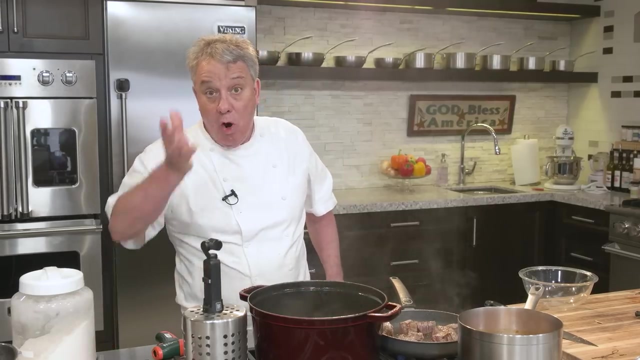 So we got our mushroom ready to go and now let me see. Let me see how we're doing here. Okay, one more thing: Mushrooms. What are mushrooms made out of? If you took my class school, you know where I'm going. right, Mushrooms are made out of what Water? 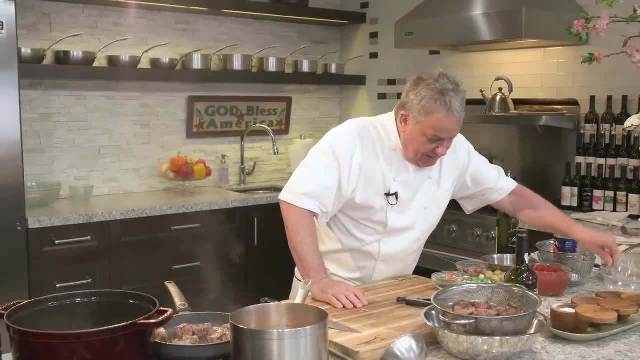 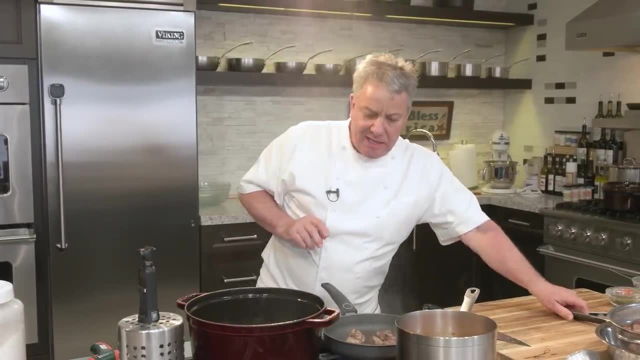 90% water. What does water taste like Nothing. So you want to keep your water in there. That's up to you. I'm not interested. I don't want an ingredient that tastes like nothing in my food. okay, Oh, look, look, Can you get that? You see how nice that is, folks. 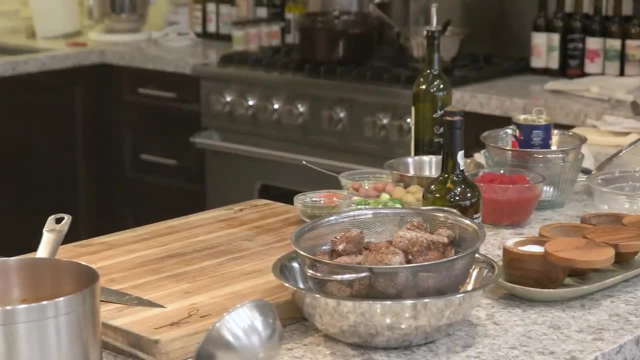 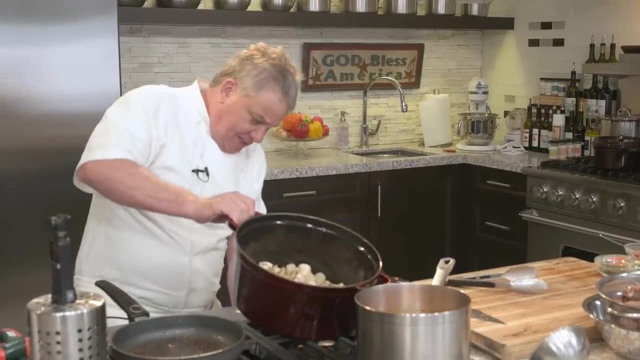 All right, so the beef is done. okay, All we did. let me just push this pot over there. I like this. I like the burner better. all right, So now. now friends, now friends we're going to get rid of. 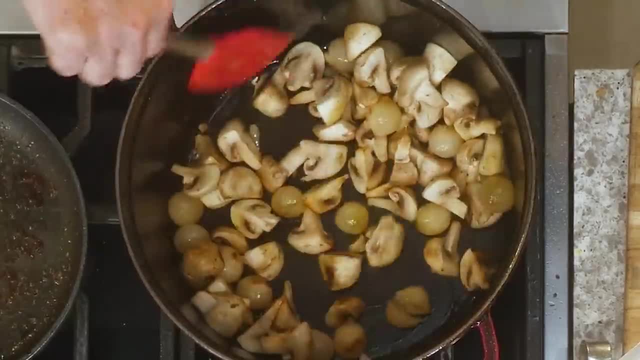 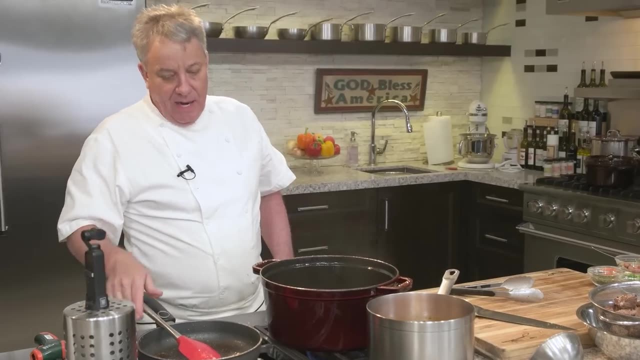 the water in the mushroom? okay, Anything with the water. I don't understand people adding water to their food. okay, If I'm going to add a liquid to my food. Oh see, like this pan though, by the way. Look, look, look, Look at this pan right there, folks See where that pan. 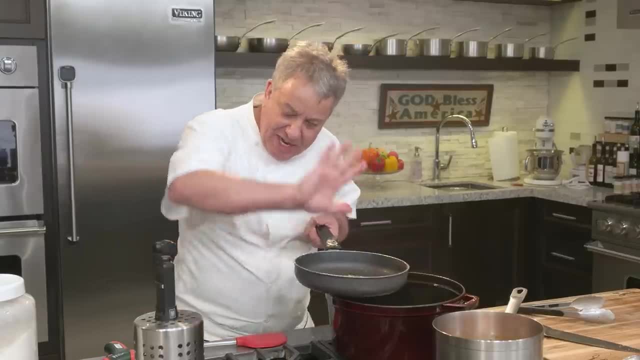 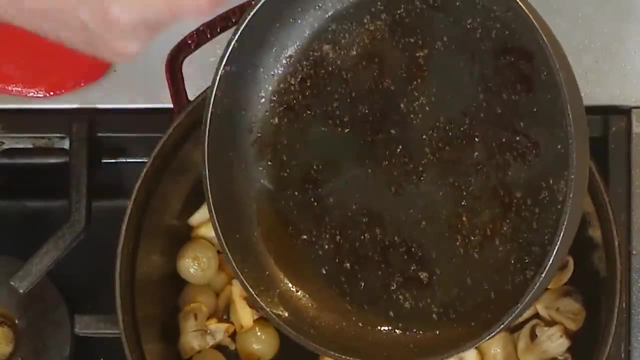 That pan right there. I got a little camera in here. It's It's full of grease from the meat. That pan right there has got some beautiful burned bits right there. So you know what I do after I'm done with it. I take my port wine and I deglaze the pan. 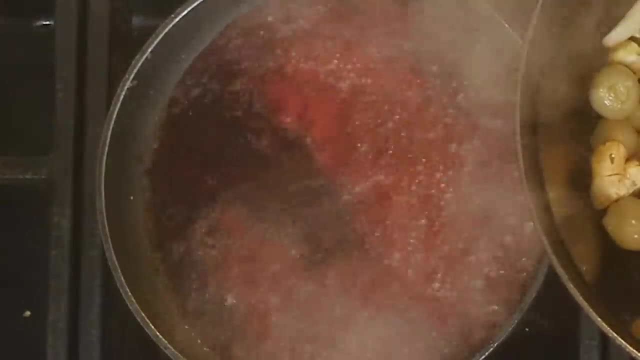 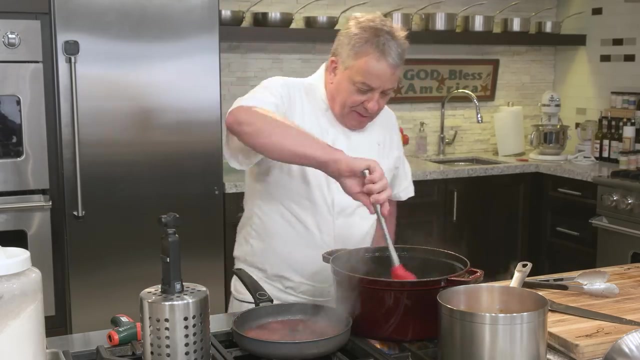 Yeah, Yes, sirree, take that pan right there and you can deglaze it, you see, And then we'll take this and we'll pour it in there, All right? So yeah, we don't want to lose an opportunity for flavor. 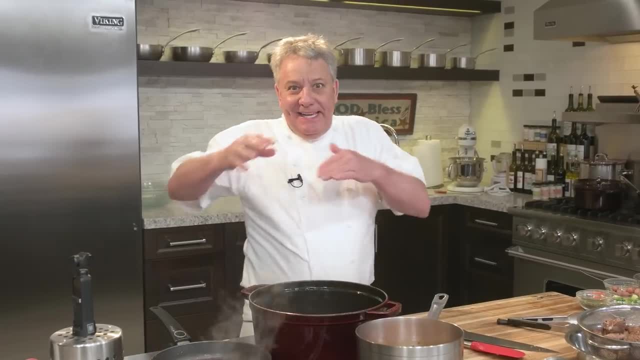 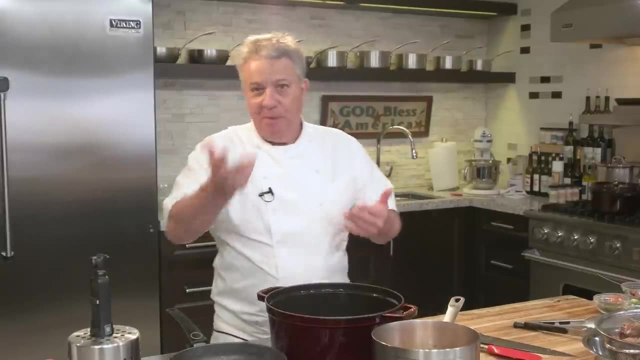 You know, to me cooking is like building a building A first story. you don't put a second story until the first one is ready, right, And you don't put the third one until the second one is ready, right, Okay, same deal. 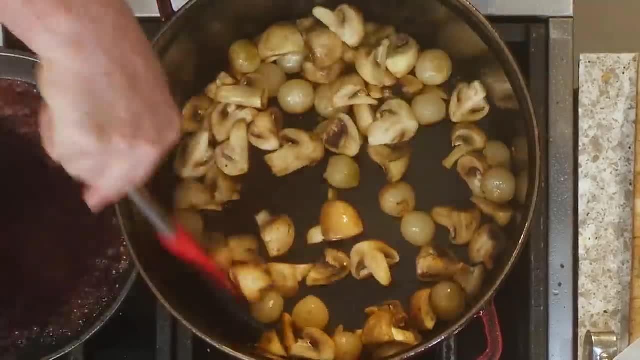 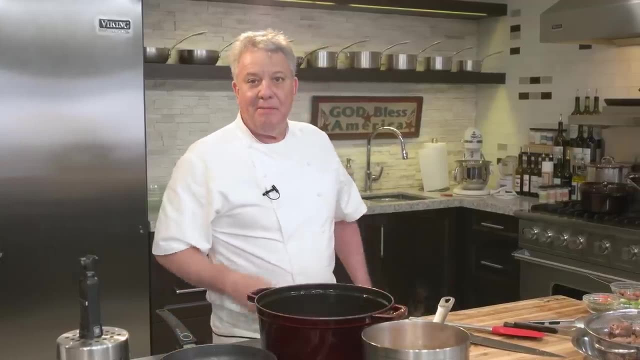 So now, look, look, look, look, I got the mushroom in there cooking and the mushrooms are going to be releasing their water. What would help them get rid of the water? Put it down there. Let's see how many of you know that. 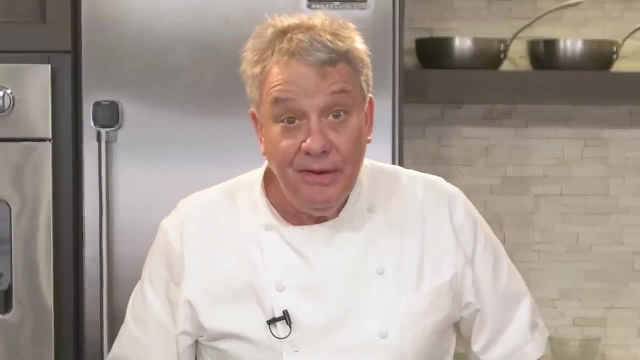 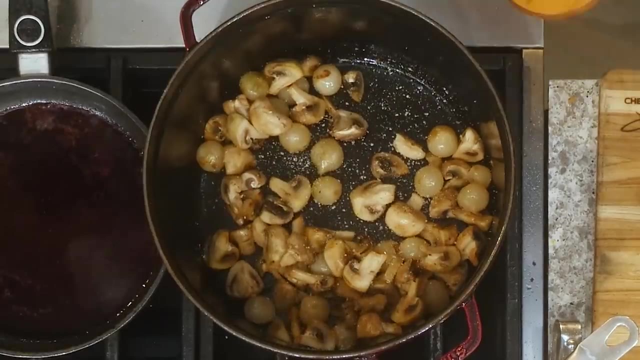 What would help me get rid of the water on the mushroom? Anybody know Salt? Yes, sirree salt. Right there, right there, I got this beautiful Mediterranean sea salt that I'm going to put on there. That's going to help me draw the water out of the mushroom. 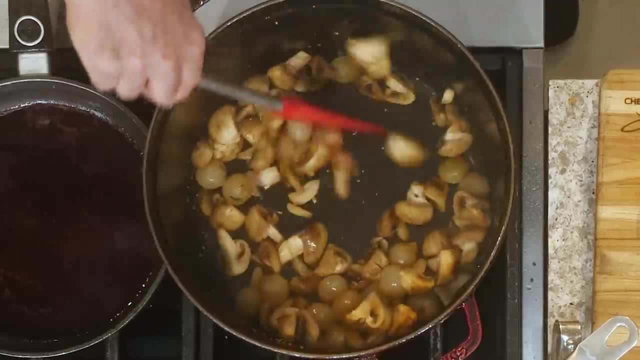 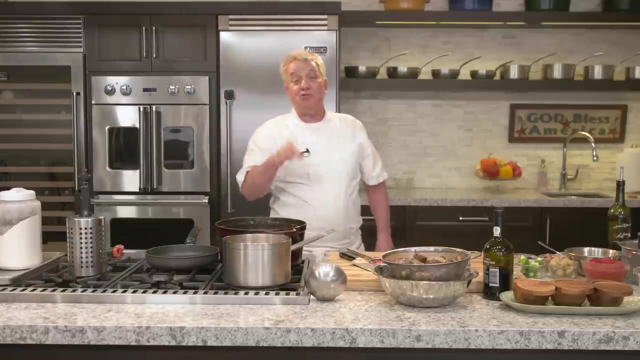 That water, the enemy. The water is not going to. You know what I find interesting? You're probably with me too with this one: When somebody uses dry mushroom. you know they use this beautiful dry mushroom. What's the first thing they do? 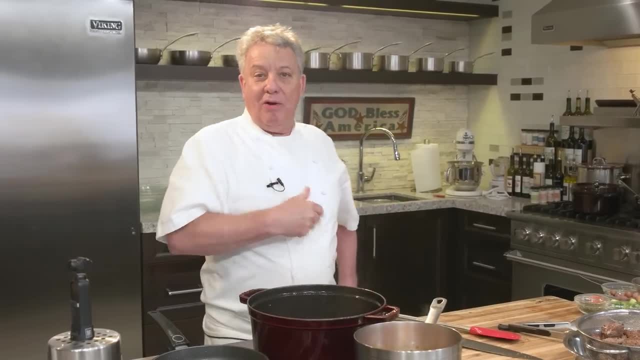 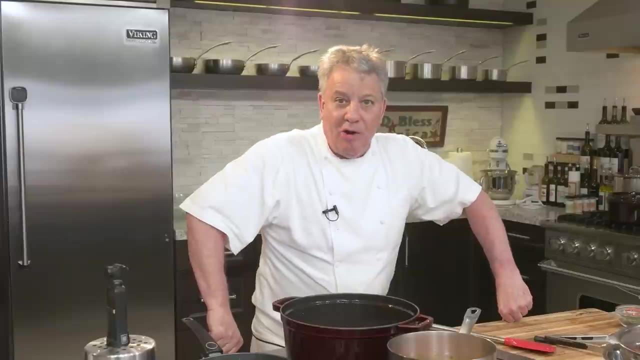 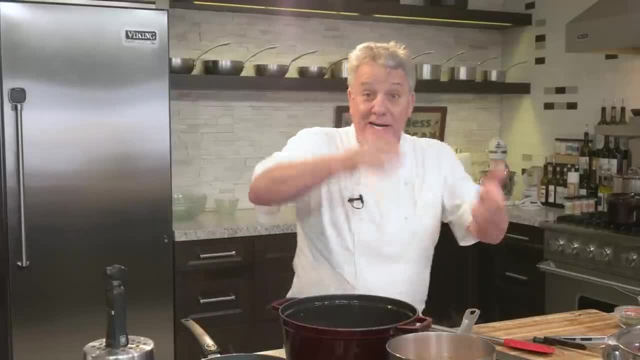 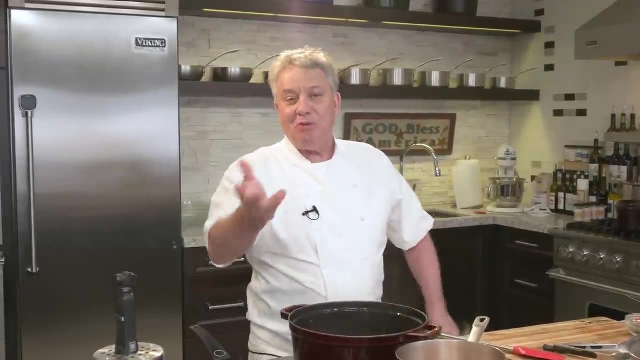 Water tastes like nothing. Put it in wine, put it in broth, put it in stock, put it in something else than water. How great is that? if you picked wine, and Let's say you picked the mushroom, and inside the mushroom is Madeira wine. 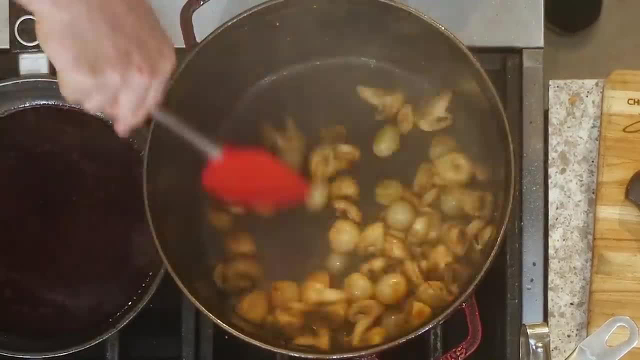 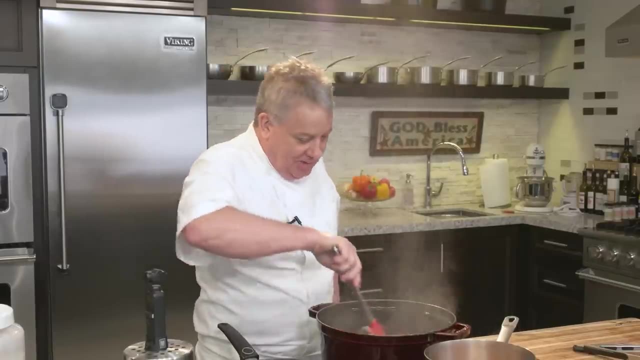 Oh, you can't buy those. But if you buy a dry mushroom and you're running from it, rehydrate them. in Madeira you got a Madeira mushroom. Well, that would be something I should do. What do you think of that idea? 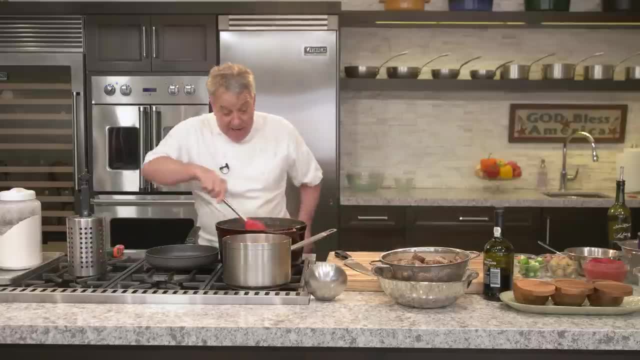 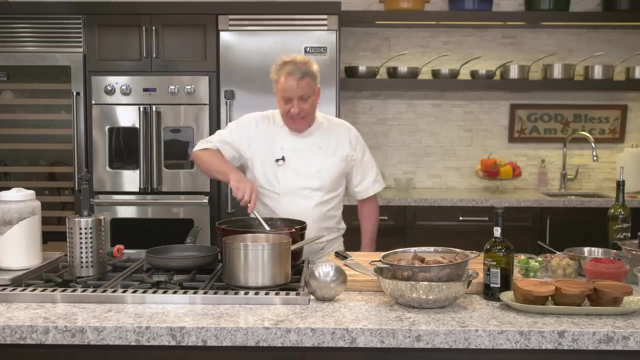 Let me know in your comment. okay, Now, if you could be here right now, you would smell- Oh, it's hot. You would smell onion and mushrooms that are not releasing their water. Now what's going to happen when they release their water? friends? 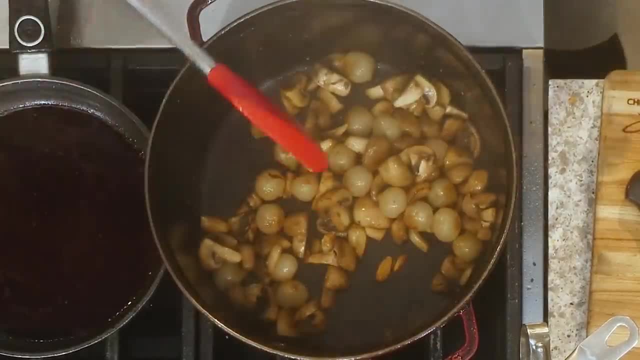 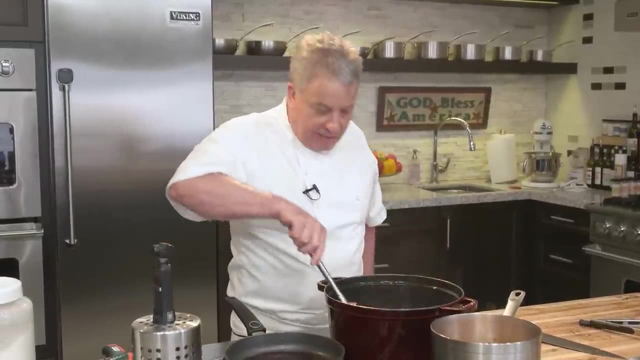 they become nice and small and that's okay. I don't need the water. Have you ever chewed on a canned mushroom? Don't do it. Don't ever chew on a canned mushroom. That will give you a nightmare. You think I'm kidding. 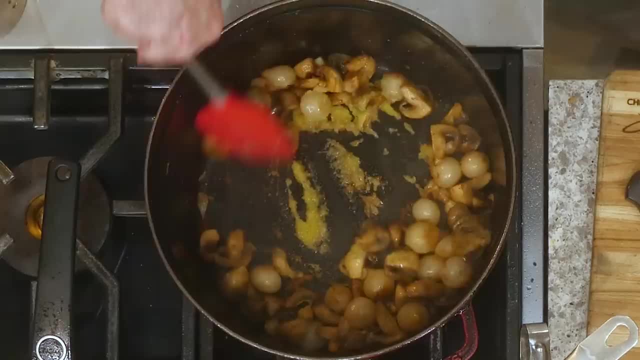 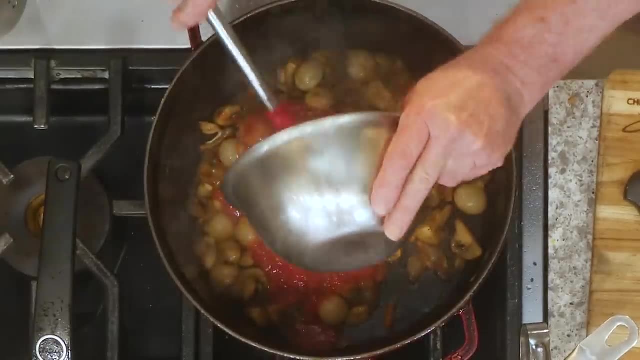 No, I'm not kidding. Now we're going to put the garlic, And as soon as you smell the garlic, friends, the second you smell the garlic, which should be about right now. we're going to put our tomatoes or anything liquid. 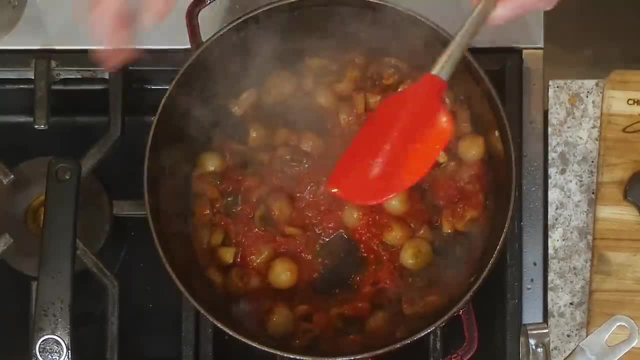 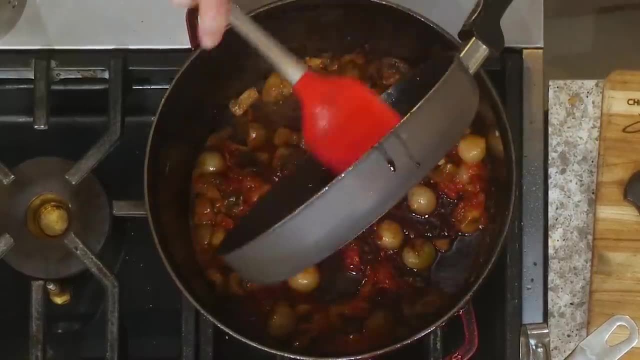 Okay, our tomatoes. I got beautiful tomatoes And then you know, I'm going to put that port wine that I got right there, that I got from the pan earlier. Add the beef in it. right, I'm putting it in there and I'm using the whole thing. right there, right. 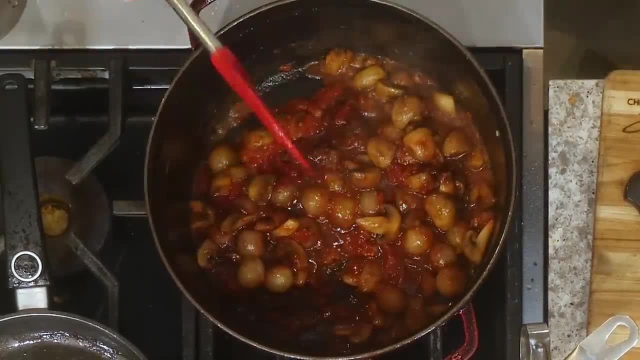 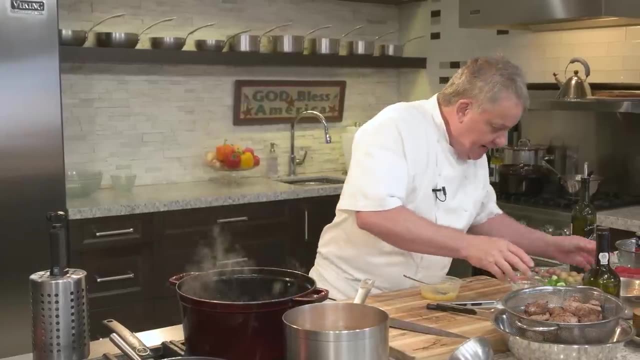 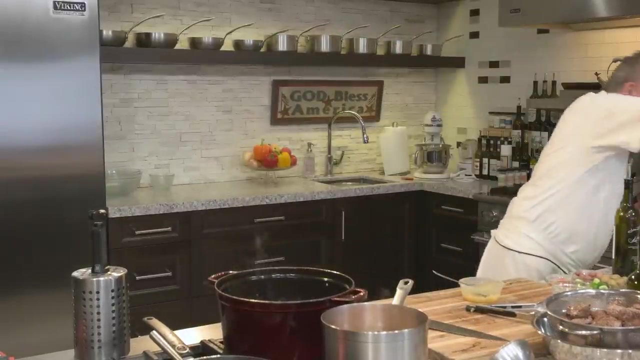 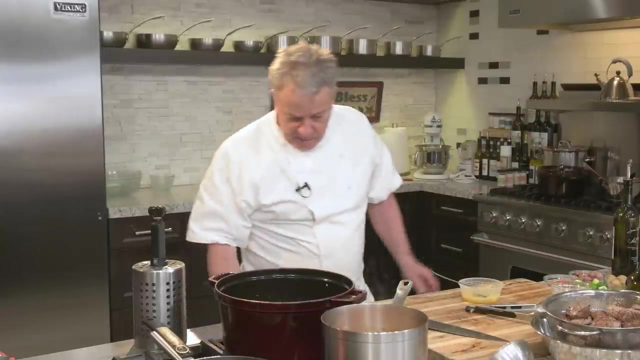 All right. So so far I got tomatoes, port wine, mushrooms, fresh thyme, fresh rosemary, little bit of tomato puree. Let me get a spoon. Little bit of tomato puree. All right, We're going to bring up the heat. 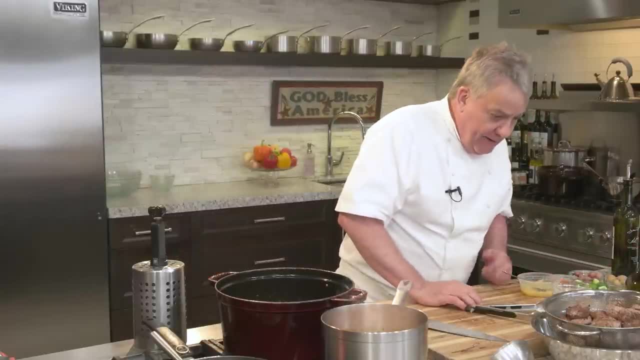 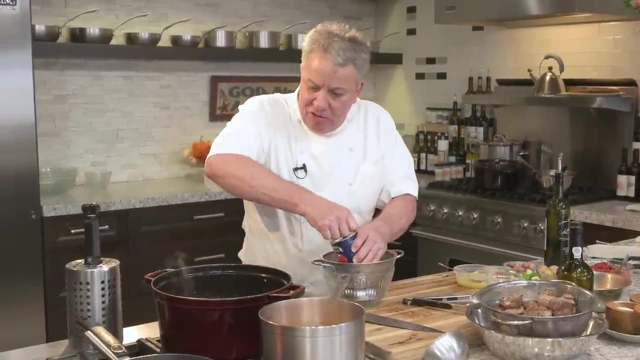 All right, It looks like it's slowed down all of a sudden. Okay, Oh, oh, oh, I got tomato puree. and you know what I got also? It's cherry tomatoes. Have you ever used cherry tomatoes? Oh, they're fabulous. 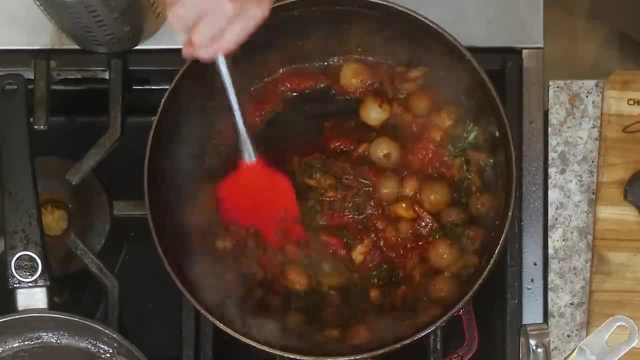 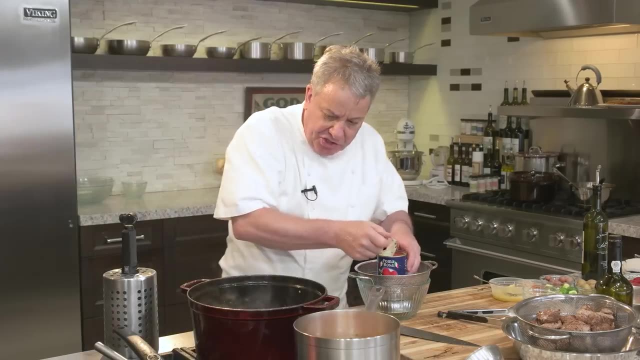 They're fabulous. Cherry tomatoes are fabulous. They give you a really, really nice texture to begin with. right, Nice texture. Cherry tomatoes, Look, look. But the problem is with the cherry tomato. can they got a lot of water in there? 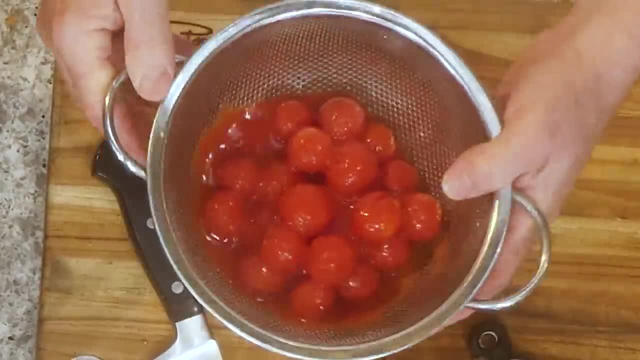 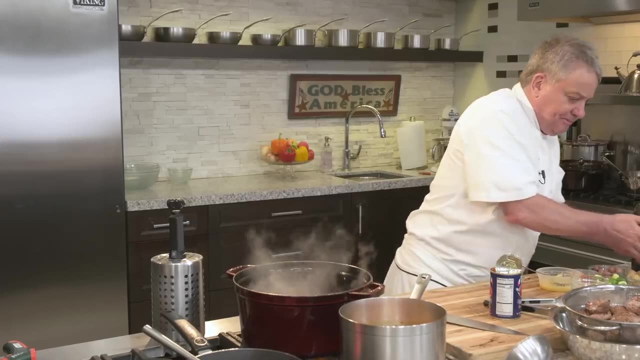 Look, I don't know if you guys can see that, but look at that. They got a lot of water, See, look at this. So I do it. Take the water out of there, Look. All right, If I want water, I'll add some. 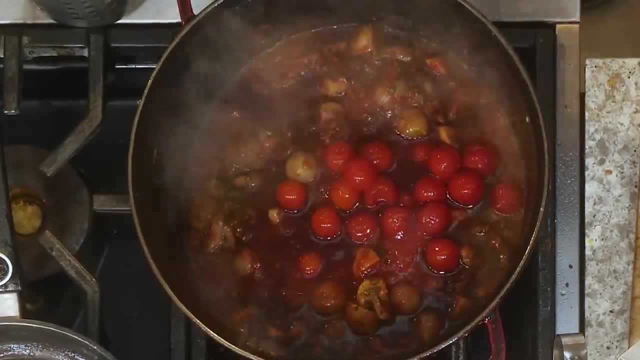 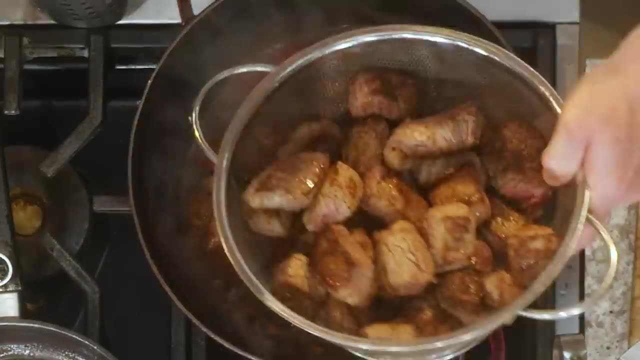 We're going to put a little more port wine. You notice everything is carefully measured, eh, Be careful. Then we're going to put the beef that we sautéed earlier. All right, So it's to save some time. 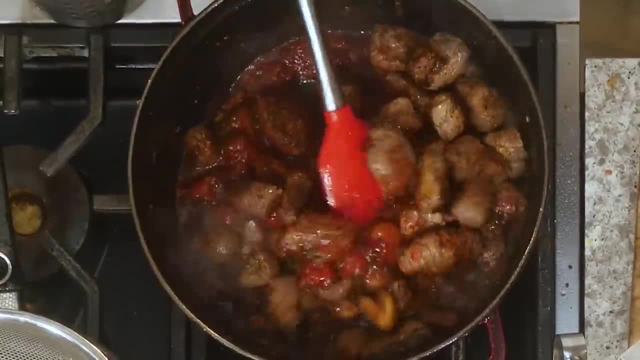 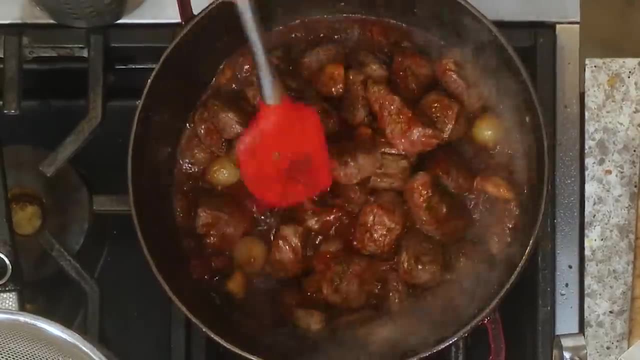 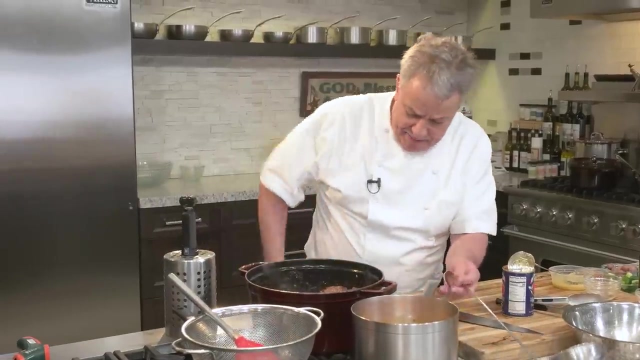 We're going to mix all this up And then we're going to put beef stock. All right, Now, I'll talk about beef stock. in a second We're going to put a beef stock. okay, All right Now, beef stock, friends, may be one of the ingredients that you don't necessarily have access to it. 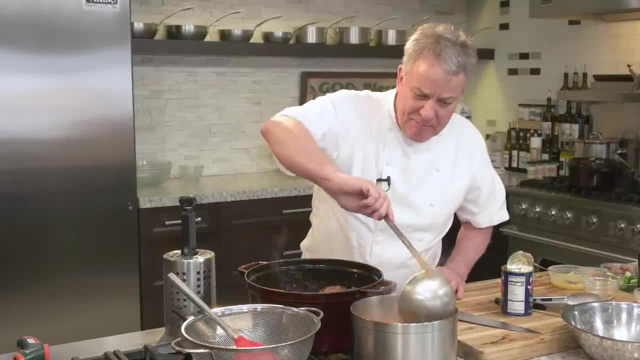 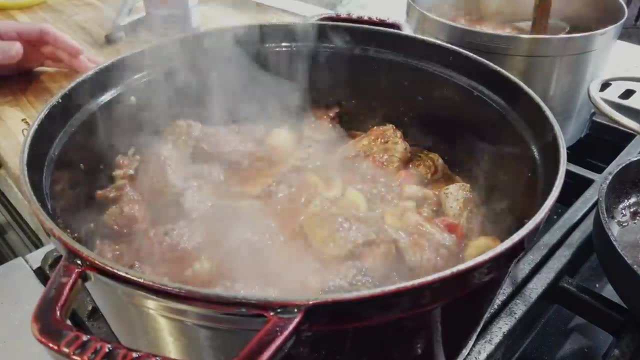 You see, Not everybody's got access to a beef stock, So what I do is we make our own beef stock. of course, because we have a commercial kitchen, It's not exactly easy for people to make a beef stock. Look. 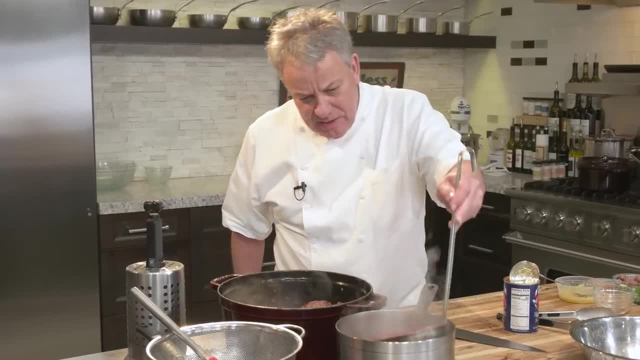 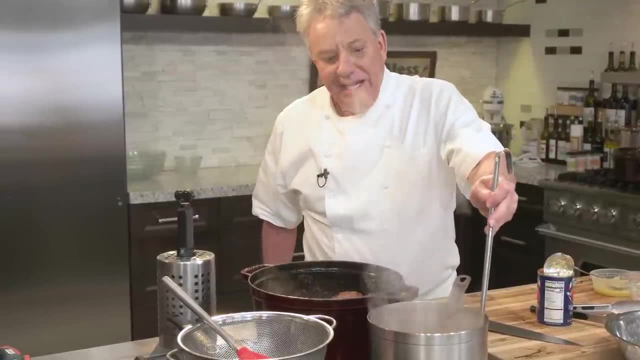 Look, Look how beautiful that is. Look at this. Look how nice and thick that is. folks Look at this. See how beautiful that is. And the reason why it's beautiful like that is because when we make it, we put tomato paste in it and we cook it for 24 hours. 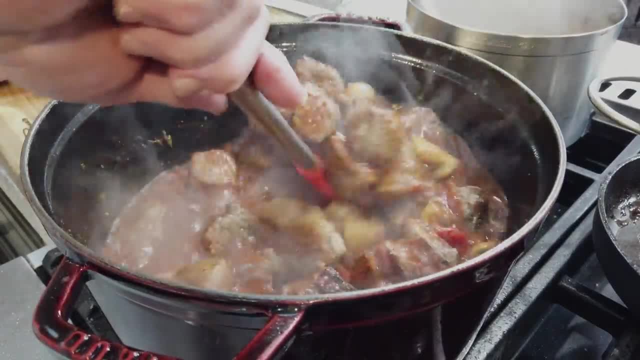 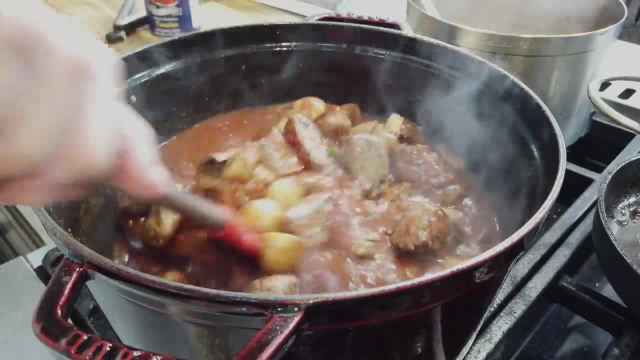 So not exactly easy to do at home, right? How are you going to make a beef stock if you're going to cook 24 hours? So see if you can find a shop that has a beautiful beef stock. If not, what do you do? 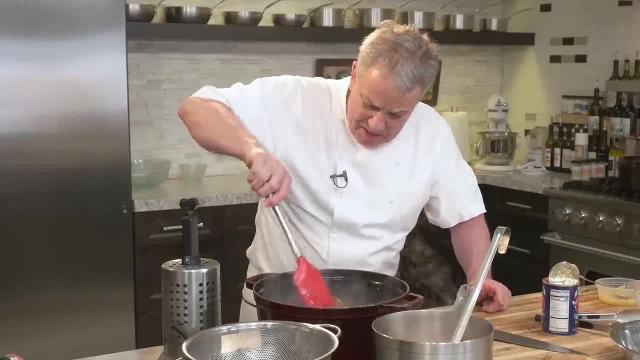 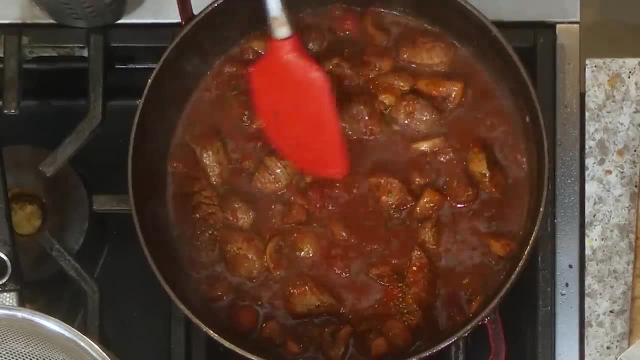 I'll tell you what you do. Oh, you're starting to look good, friends. I'm telling you, I'm coming back here more often. The food is delicious. Let me tell you what you do, friends. You get yourself a, and you know what we're going to add to this. 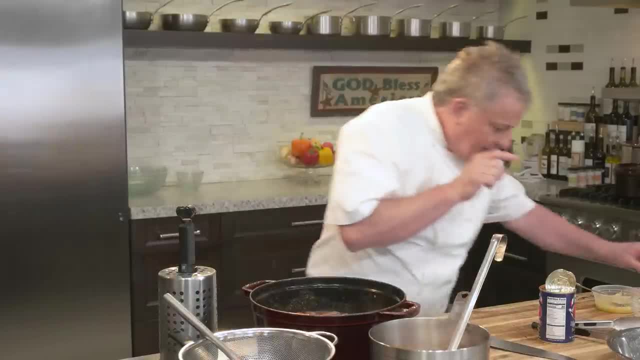 We're going to add some. I got those baby potatoes, Look, look, look. I got them cooked already. I'm going to finish them up. Look, Look, how cool they are. Little baby potatoes, All right, Little baby potatoes. 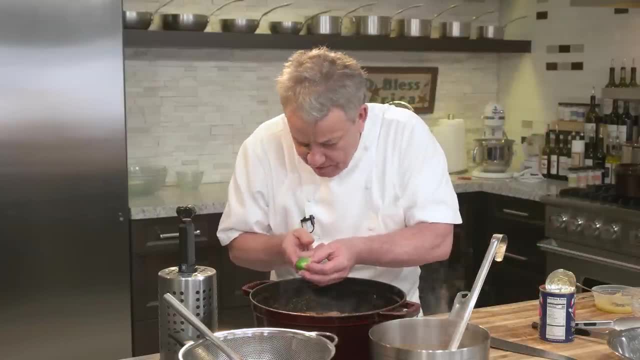 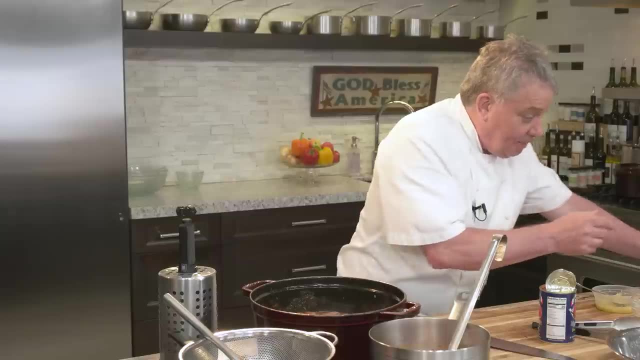 And I got those baby Brussels sprouts. I already poached them. And then I got those little baby carrots. Look how small they are. So I sauteed them, I sauteed them, I sauteed them, I already poached them. 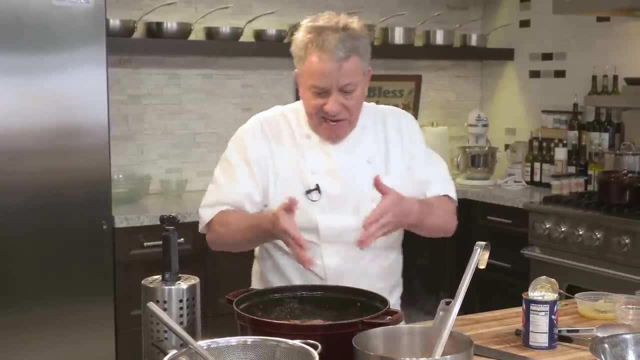 So they cook right. So I'm going to saute them in butter. I'm going to add them at the end, Because if I add them down they're going to fall apart. This guy's going to cook, This is going to cook for two and a half hours. 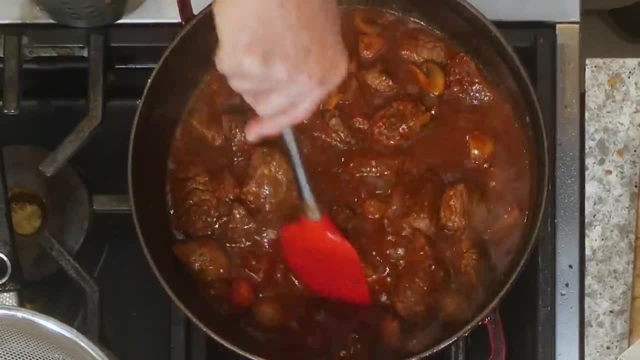 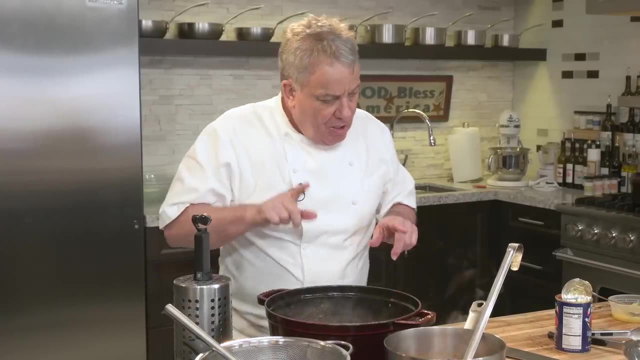 This is ground chuck. You want it to really, really really be tender. You got to cook it for two and a half hours at a very, very, very low heat. Okay, That's the secret. Okay, So where was I? 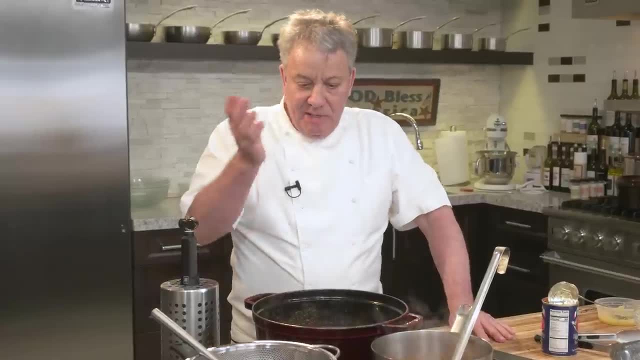 Oh, oh yeah, Sometimes I lose track of what I'm talking about And there's nobody here to remind me. So, to go back to the thing, But I was talking about a beef stock, So what are you doing? 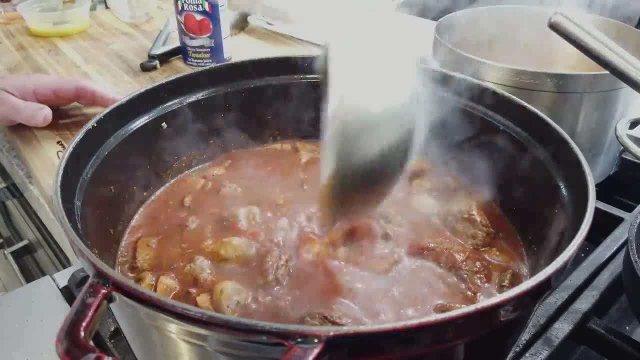 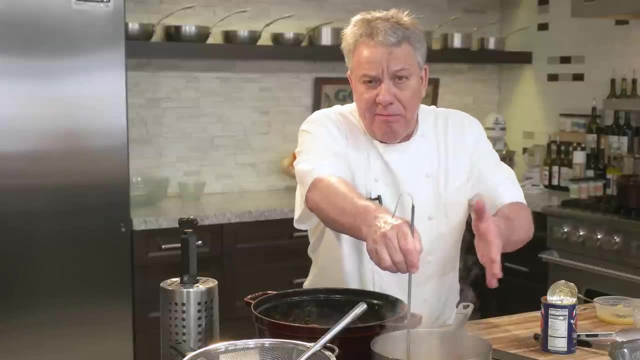 Well, you buy a good beef broth. Buy a good beef broth And add some tomato paste to it. If you have some extra leeks, carrots, celery and onion, add it to it And cook it for a little while with the tomato paste. 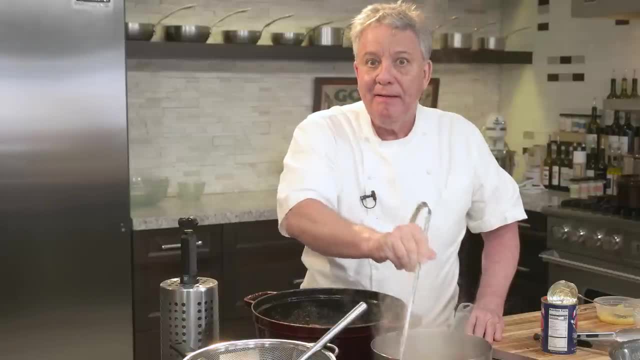 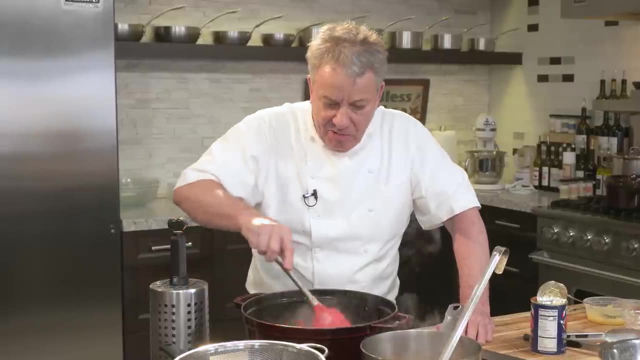 And look, It's going to give you a rich consistency like this And you can keep it in the freezer for 17 years approximately- Don't quote me now. I can see people going 17 years. You know what we got with YouTube. 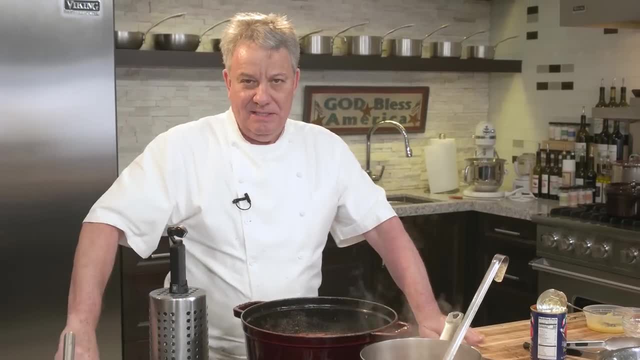 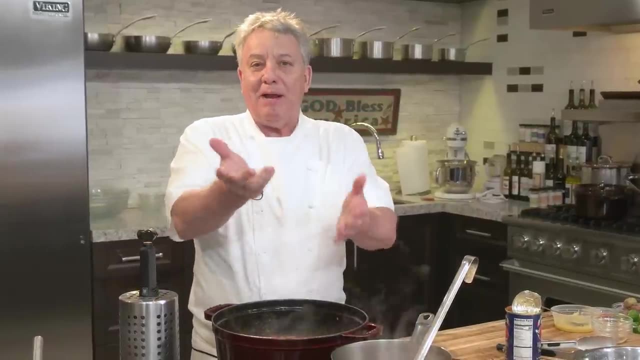 We're good, We're lucky, We got recipe police. I love it. I got this thing where I do a recipe on peeling a tomato Tomato con case. I'm showing people how to make a tomato con case. I'm putting it in the water. 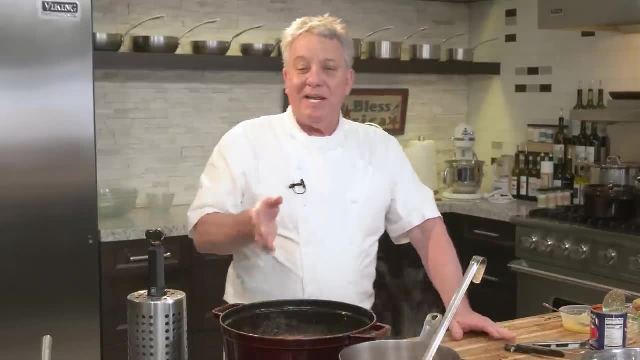 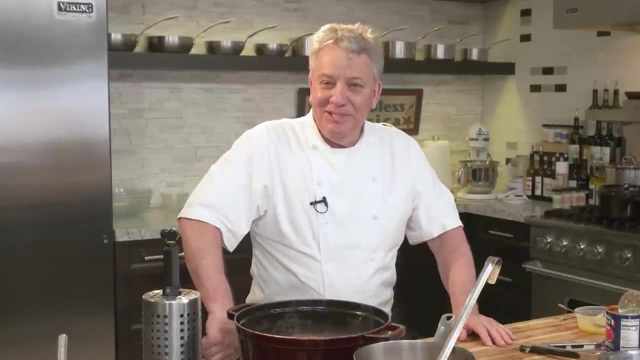 And I said it should take about 10, 12 seconds. You know how many of them said: oh, it took 23 seconds. It took 23 seconds. I'm glad they got a better clock than me Now. they got better things to do. 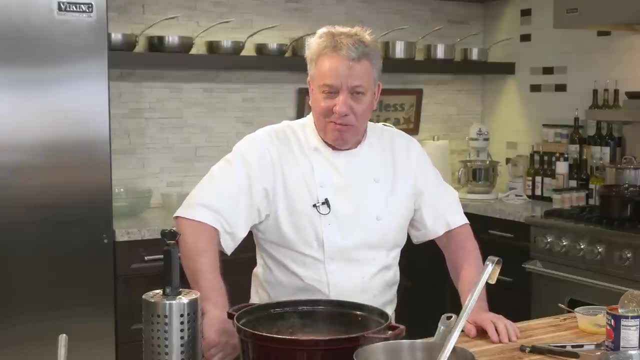 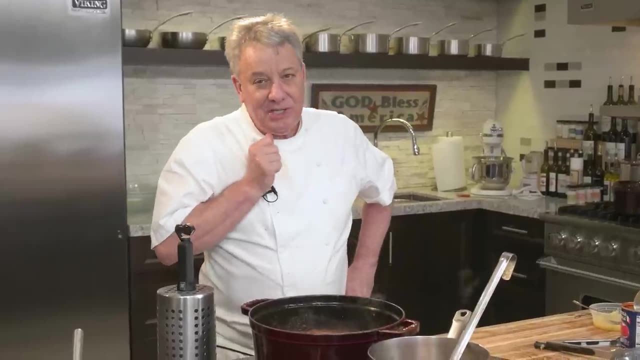 Oh my goodness, He said 12 seconds. It's 23 seconds. What's wrong with him? Don't you have better things to do, Jesus Christ, Anyway. So look, Now let's talk about thickener a little bit. 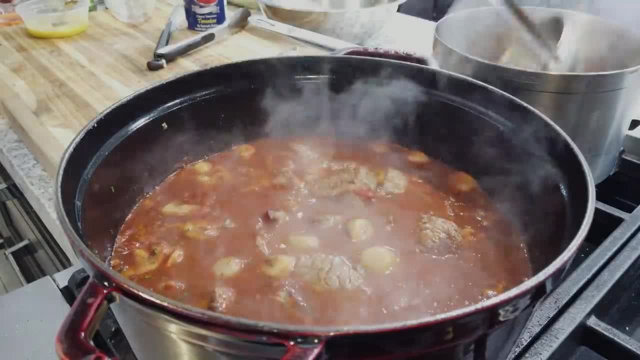 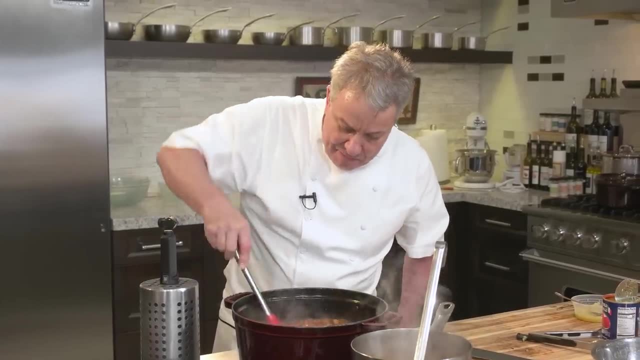 You know I like my beef to be a little more beef stock. Okay, Well, why am I putting more? You're wondering What's the matter with him. Well, because I like it to be submerged. I like my beef to be all submerged. 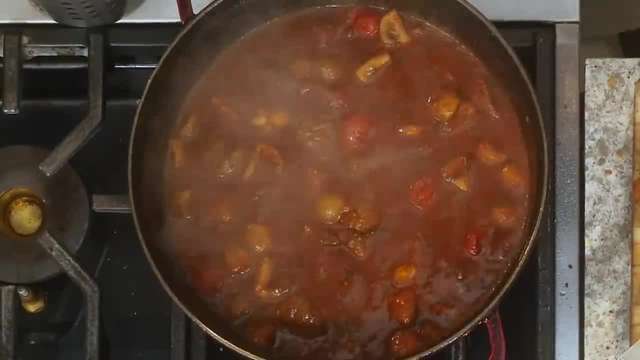 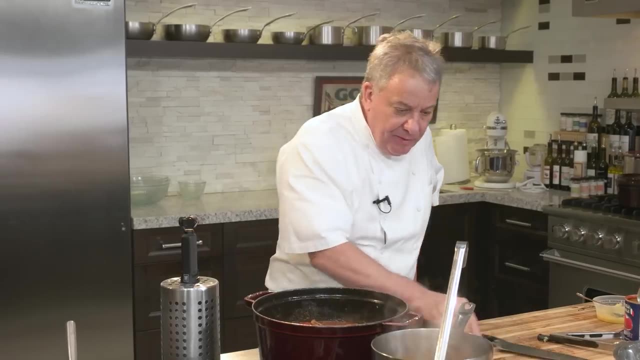 You see, All right, Submerge. You know what that means, right, Submerge Like you're submerging it. All right. So now Flour, Flour. I could have put flour when it was dry, Right. 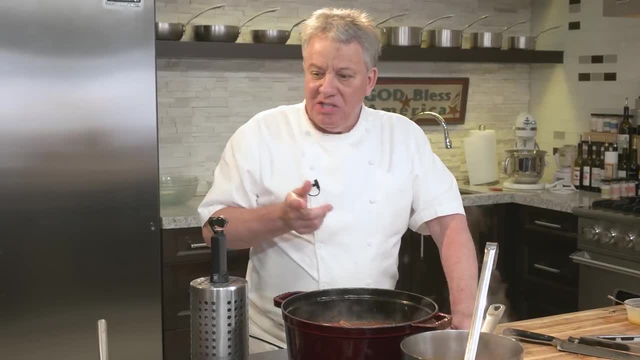 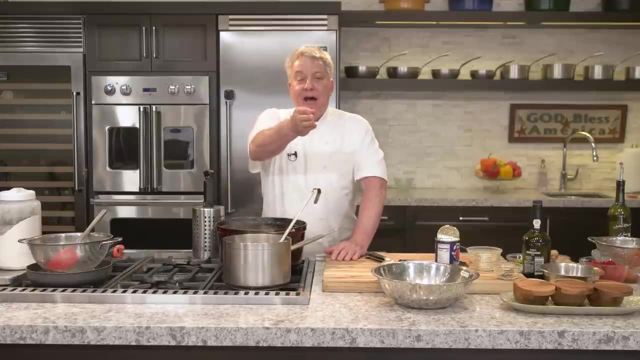 Dry beef And you put it on there. A lot of people do that. I think it's okay. I got a much better trick. though Pay attention, I'm going to teach you something. You want to thicken something, By the way. when do you put the flour? 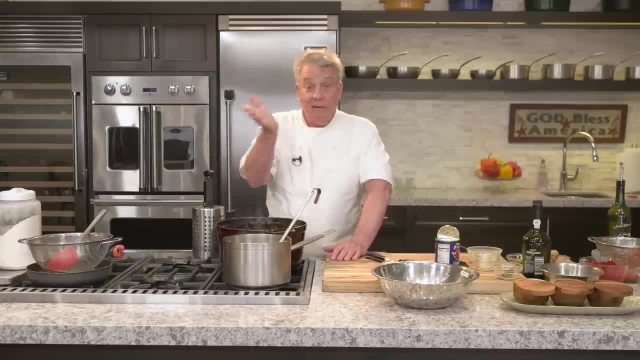 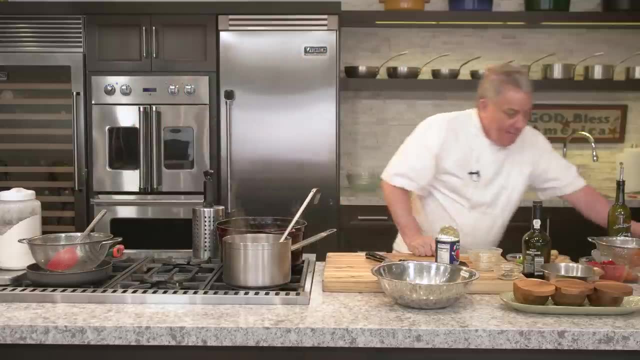 At the beginning or at the end, Beginning or the end? Beginning or the end? Huh, Nobody knows, Yeah, Unless they've been to my class. If you've been to my class, you know Beginning: The flour goes in at the beginning of the dish, not at the end of the dish. 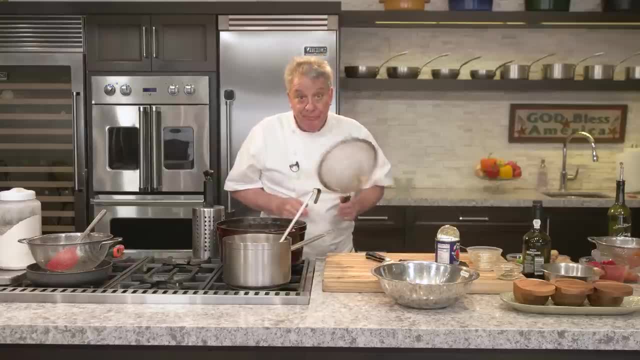 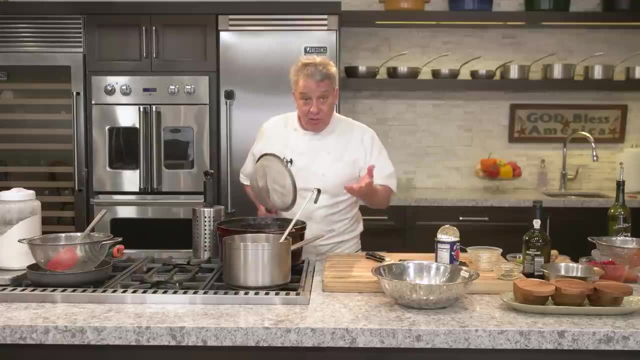 If you put at the end of the dish it tastes like glue. Yeah, Glue. You know, when I was a kid we used to make stuff with flour and water, Glue them together. We used to. It was glue. 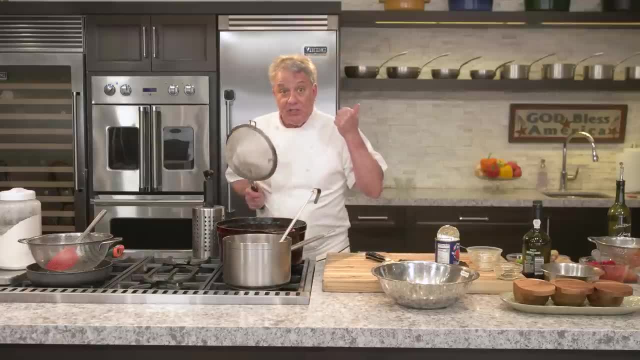 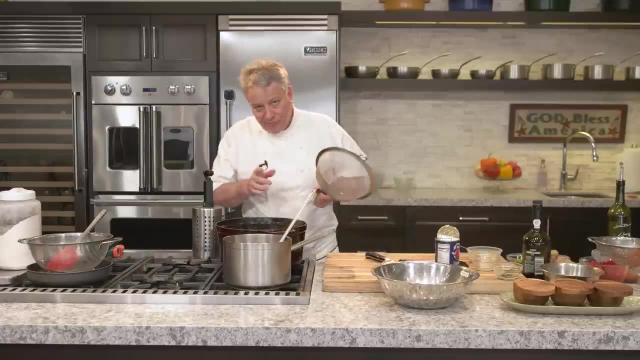 The stuff I glued 50 years ago is still glued up. Okay, So when you eat raw flour it's in there And it takes a while to get rid of it. You know I always explain to people Thanksgiving dinner. 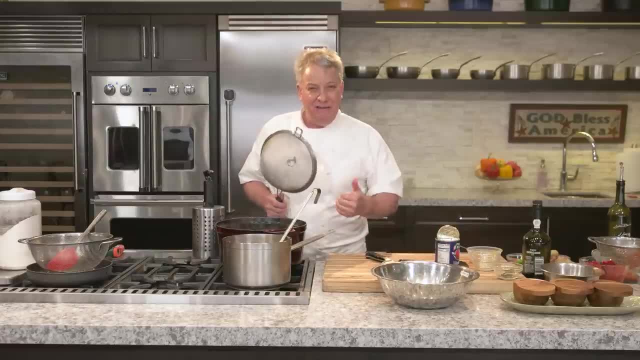 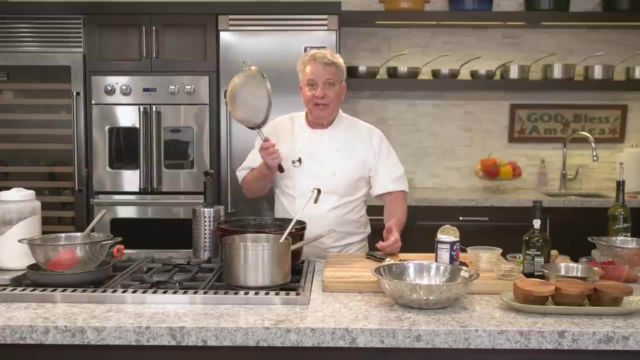 Most people. they take the dripping of the turkey right, That turkey Fat Crap, And they add flour to it And they give it, And they give it to their guests. And what do they do after they eat the Thanksgiving dinner? 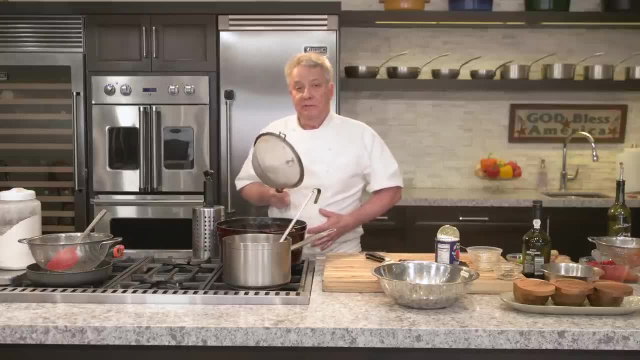 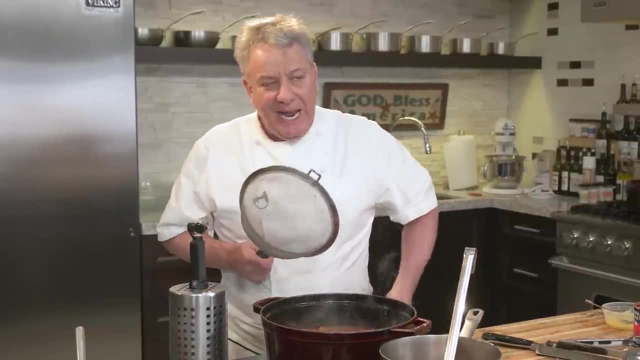 They sit on the couch and they go. I can't move. I can't move. I ate too much turkey. There's not enough trictophan in five turkey to put you to sleep. It's the glue you just consumed. Okay. 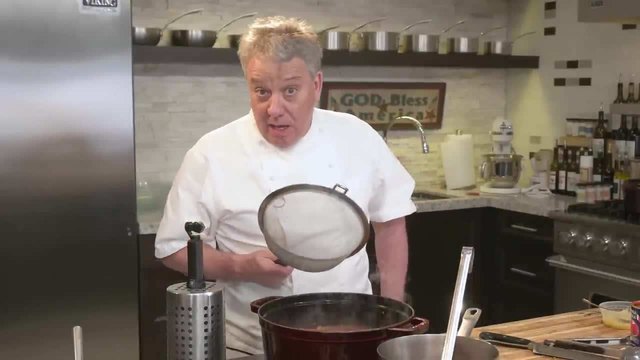 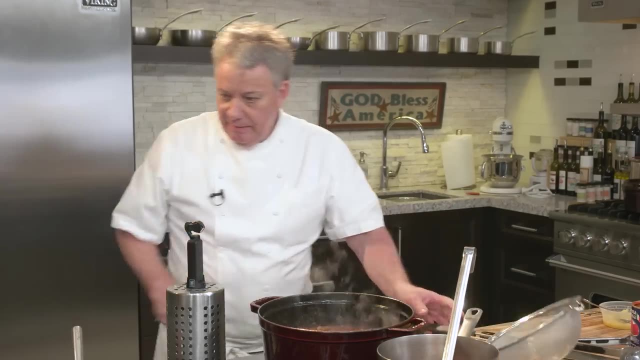 You consume turkey fat and raw flour. Yeah, good luck getting up the couch, Anyway. So, look, I was going to show you a trick. The flour, Okay, Look, look, look, look, look, If you've been to my class. 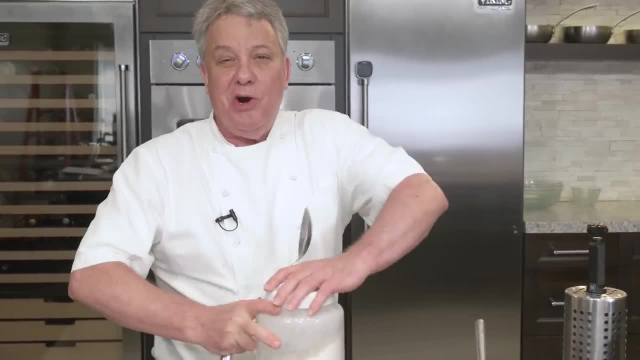 if you've never been to my class before, you're probably laughing right now because you know where I'm going. But if you've never been to my class before, you're going to wonder. So I'm going to put the flour in here. 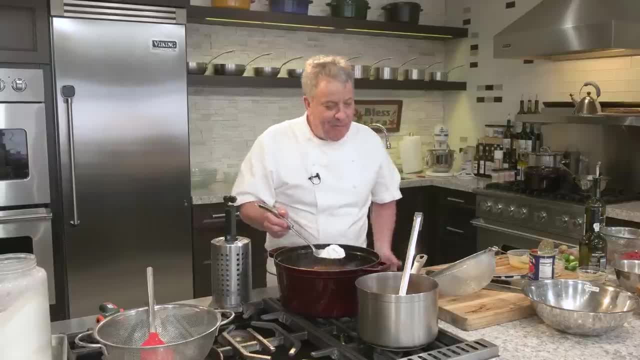 See how many of you reacted already. You don't put it in here. If you put it in here, well, I'm going to have a huge mess, right? So pay attention. Look, look, You take the strainer. 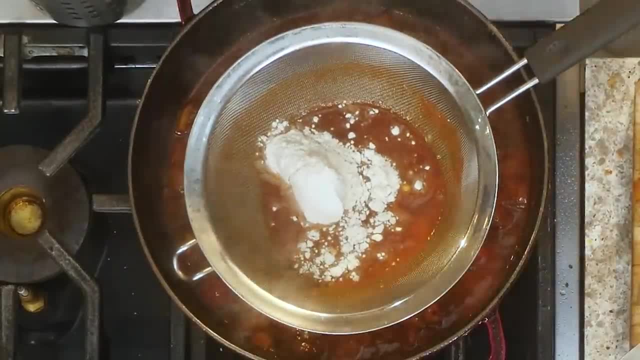 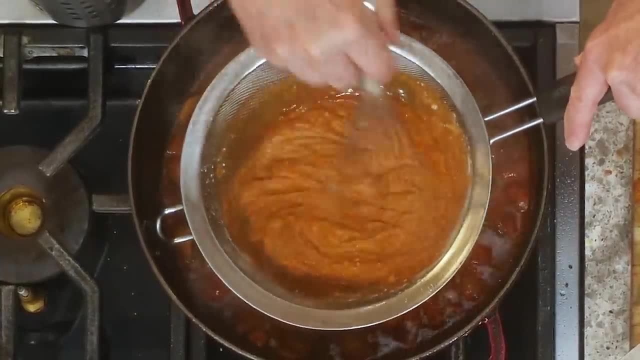 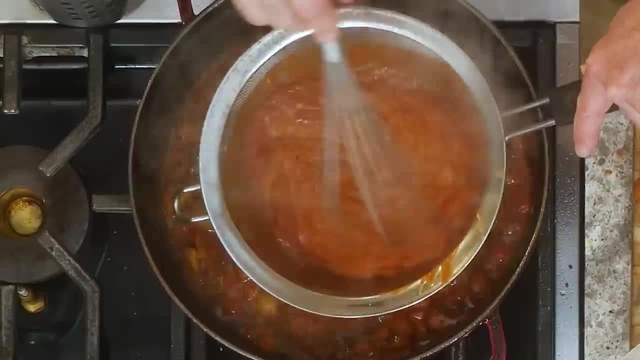 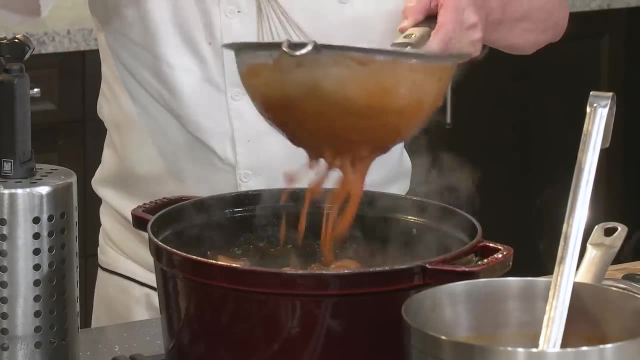 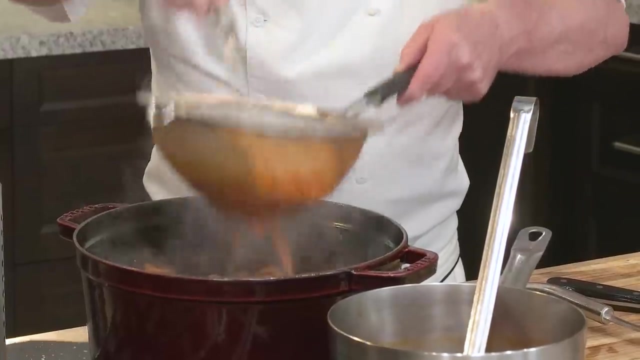 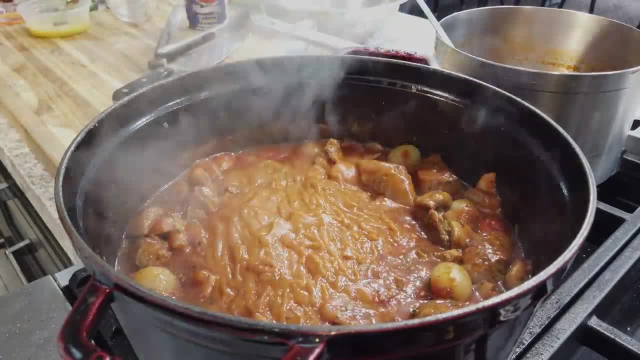 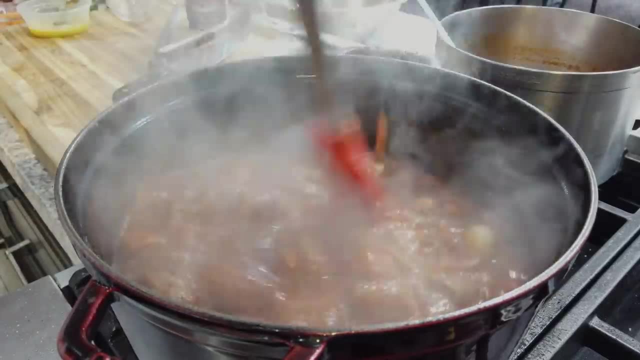 Because you don't remember. Let me just use the spatula right here. We're going to put it in. We're going to put it in. You see, See, See, See, See. Now let me tell you something, friends. 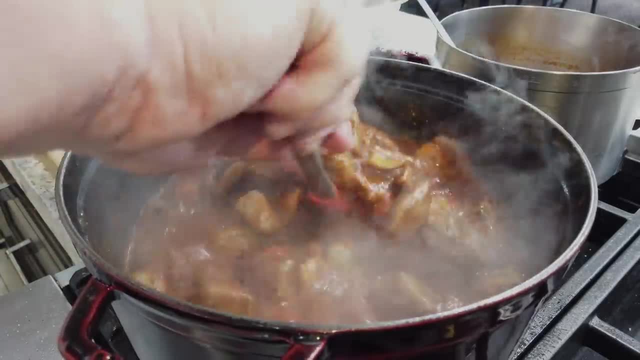 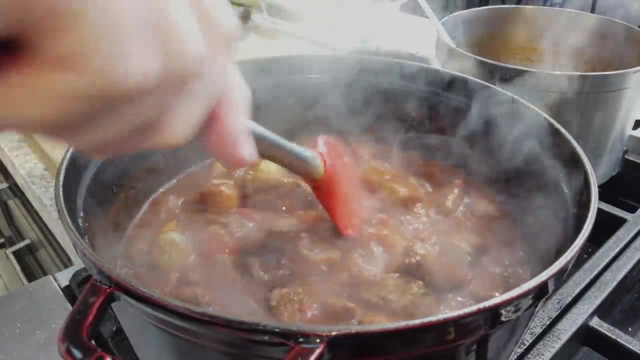 When you have a soup, a gravy, a sauce, then you want to thicken. Now, remember, you can't do that at the end. Now don't be doing that Thanksgiving deal I was just telling you about. Don't be doing that. 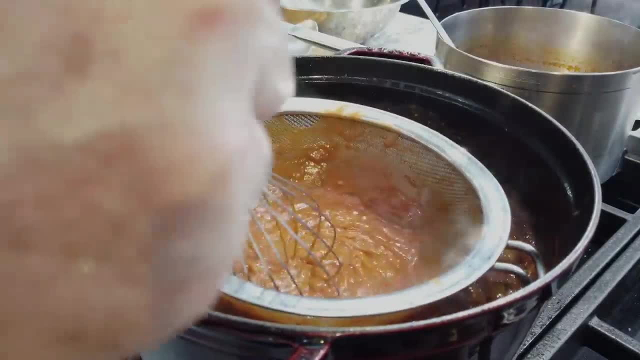 Mm-mm-mm. That is not working. So now, look, We'll go back and put a little bit more. Maybe I'll put just a little bit more stock On top of it. I want to get rid of it all. 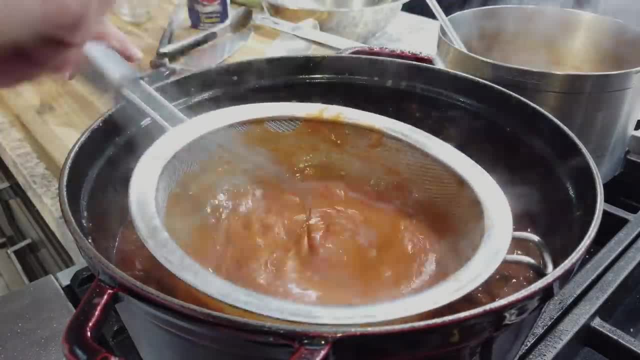 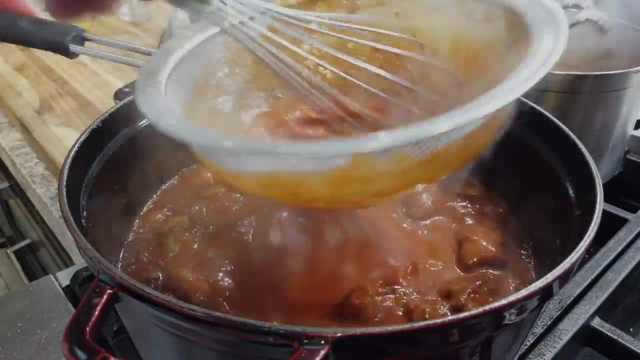 You see, Look, And then we're going to mix it up Now if at the end, All right, look, See, Look, No lumps, None whatsoever. It's the easy way to do it, But you have to use the double mesh strainer. 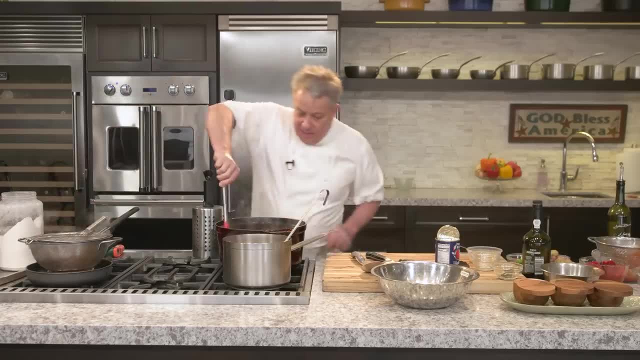 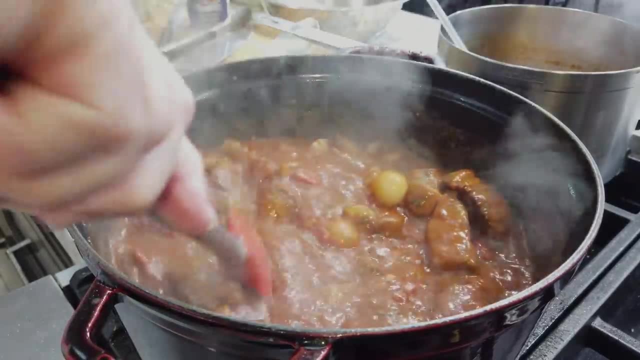 Very fine strainer, Right When you do this And you mix it up, You see, Look Now if at the end, because the tomatoes are going to release more water, you know we're not at the end, right there, you know. 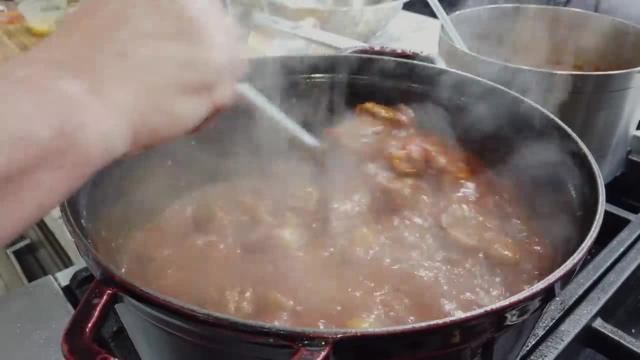 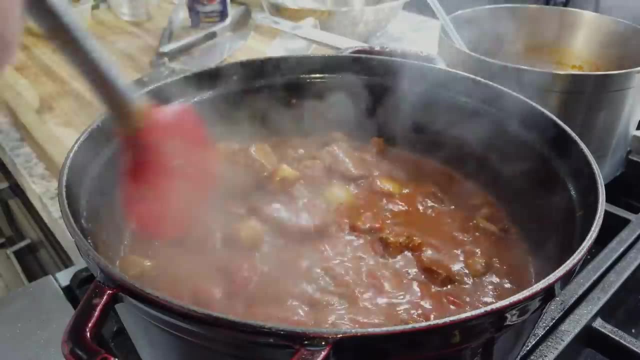 So it's very possible that we need more flour, Because I didn't put that much flour at all. Okay, It's very possible that we need more At the end. we won't be able to add any more flour because it has to have time to cook. 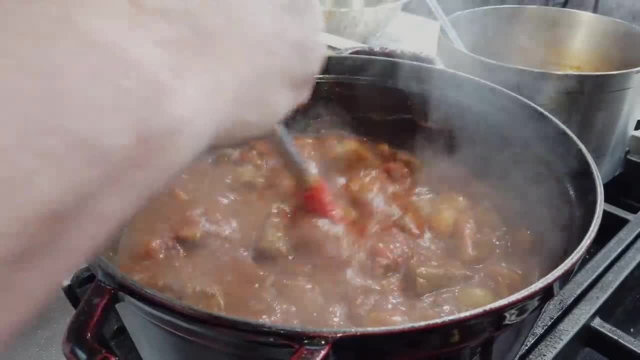 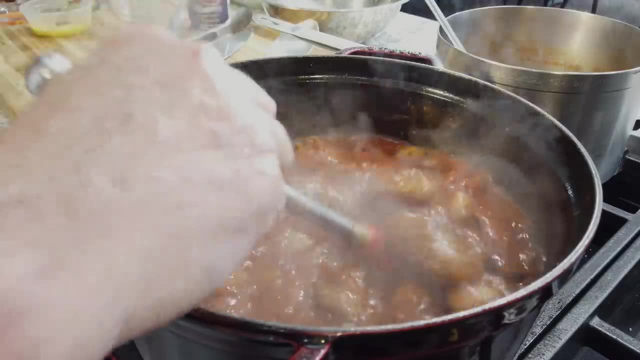 So I could use. I could fix the consistency with a little bit of cornstarch at the end, But flour of course. Look, If you're a professional cook, you have a roux, You have a cooked roux. 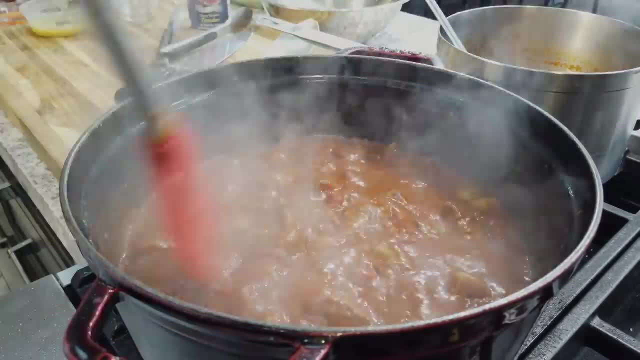 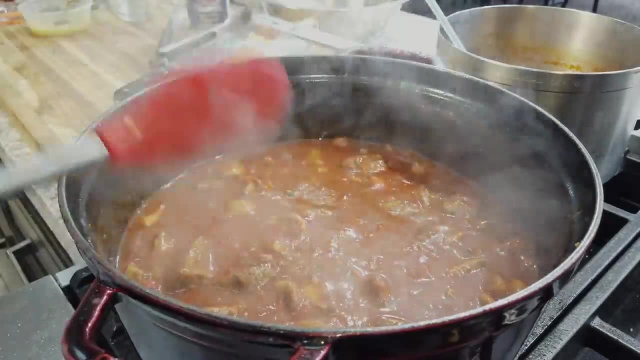 You can put that in there, But most people don't have a cooked roux. Trust me, I know That's what I do for a living. I teach people. Okay, This is my thing, Okay, And I know that most of you don't have a cooked roux at home. 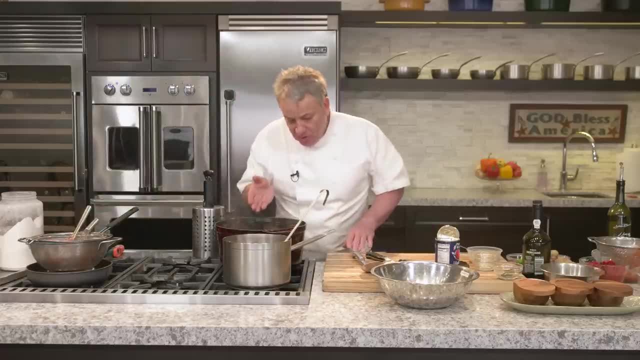 So you need to thicken, And this is a perfect way to do it. So we're going to let that cook very slowly. Bloop, bloop, bloop, bloop, bloop, bloop, bloop. 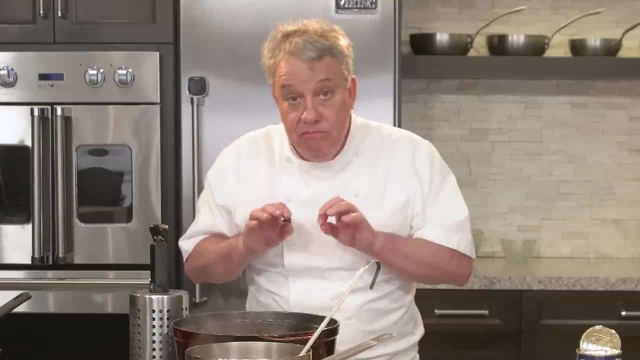 Very slowly. Yeah, Not bloop bloop, bloop, bloop bloop. That's no good Bloop bloop, bloop Very slowly. Right, Let it cook. We don't cover it, We just bring it to boil. 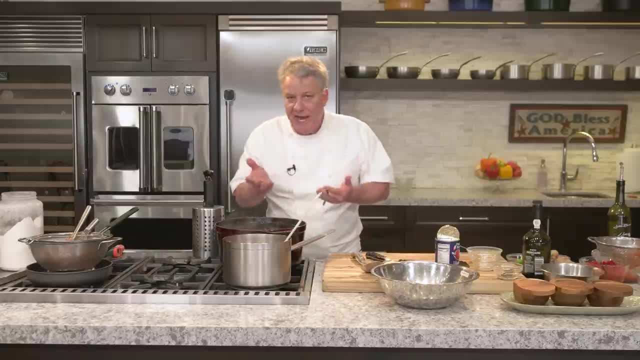 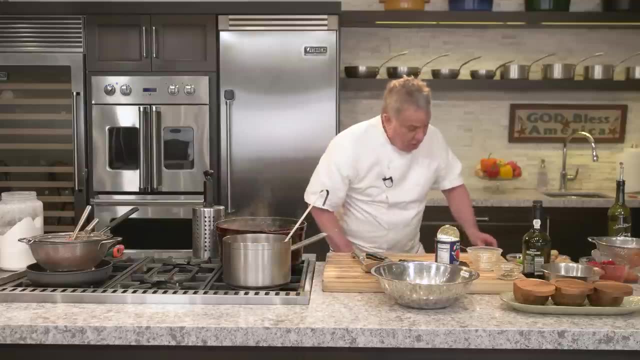 The minute it's boiling, you reduce it, Let it cook Two, two and a half, three hours. Depends, Depends, Depends on your meat. You'll know When you take a. you know how I do it. I take a wooden spoon. 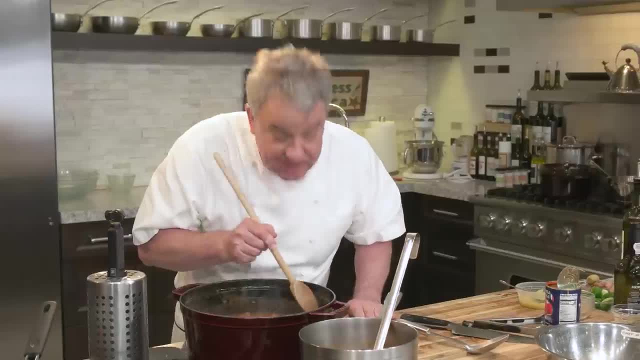 Right there, right, And I go in and I take a piece of beef and I put it on the side And if it starts to fall apart, then I'm going to test it. I know it's going to be almost ready to go. 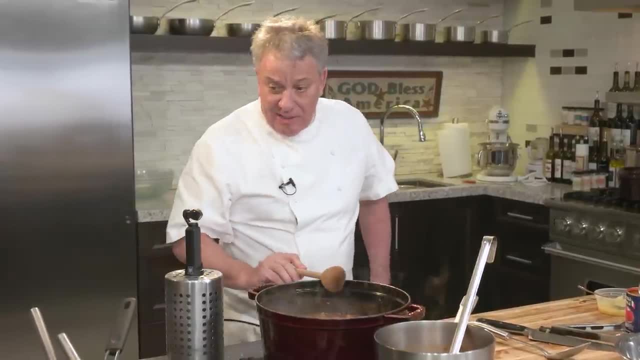 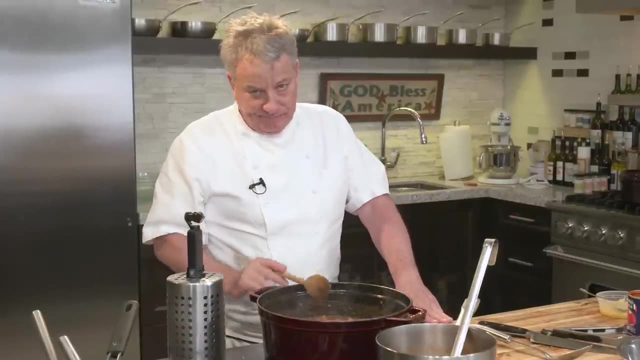 We season the salt and pepper till the end and we're done, We're ready to go. Let me tell you something: This: with our mashed potatoes, all the vegetables added, amazing Make extra because the frizz is beautiful. I'll be back when it's cooked and we're going to serve it. 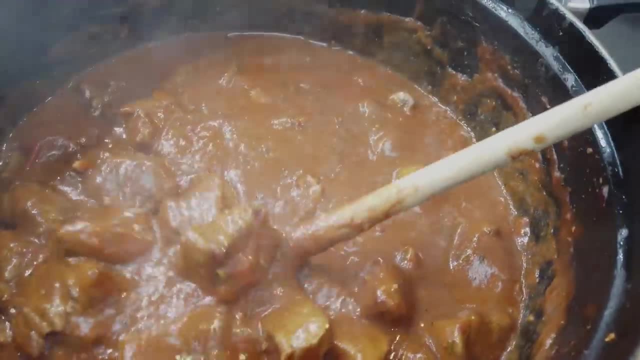 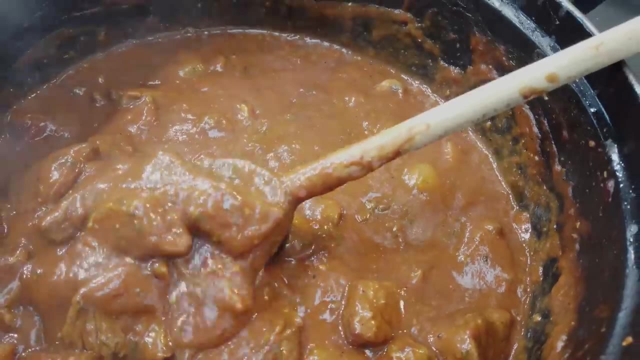 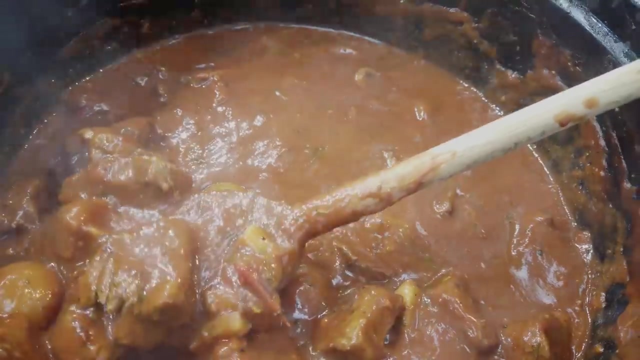 All right, friends, We're. two and a half hours went by. It went so fast, especially for you guys. And this is cooked And I want you to see the thickness of the sauce. You see, It has to be covering the beef right. 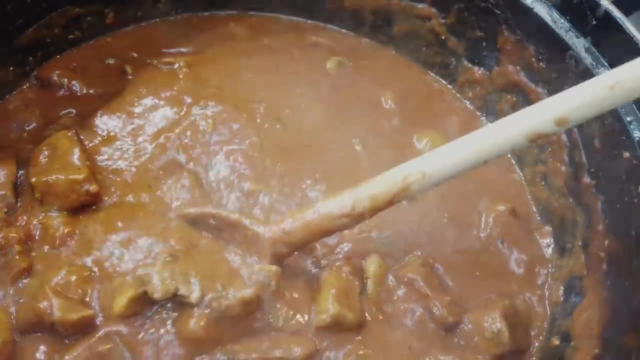 So you see, look, there's sauce on the beef. If it was too liquid it wouldn't be on the beef. It's kind of like when I make a gravy for Thanksgiving, I want it to stick on top of the turkey. 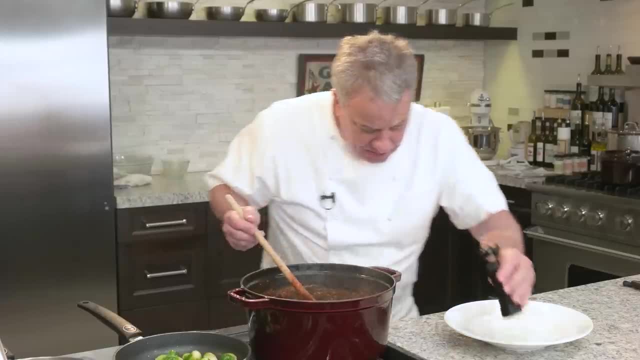 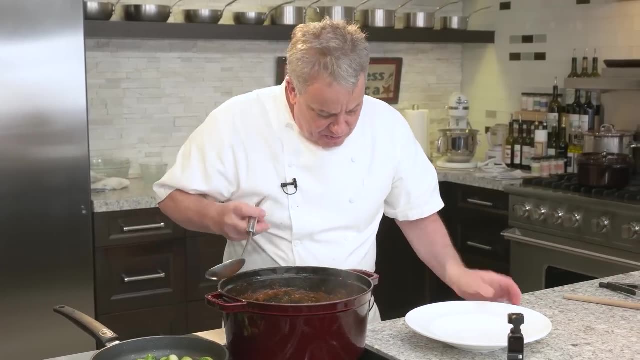 Same deal here. you see, The sauce is on top of it. So all we're going to do, we're going to plate it And all I'm going to do is I'm going to take my serving spoon And I got myself I love those big, big plate, big serving plate like this. 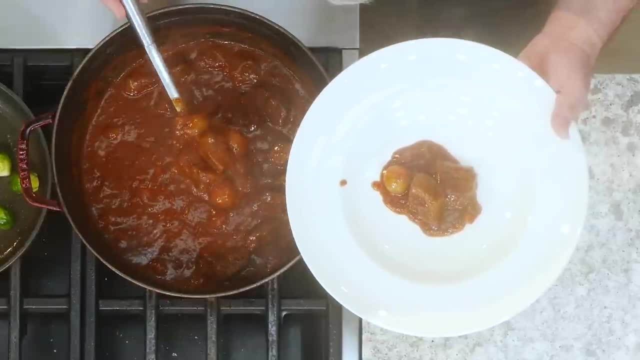 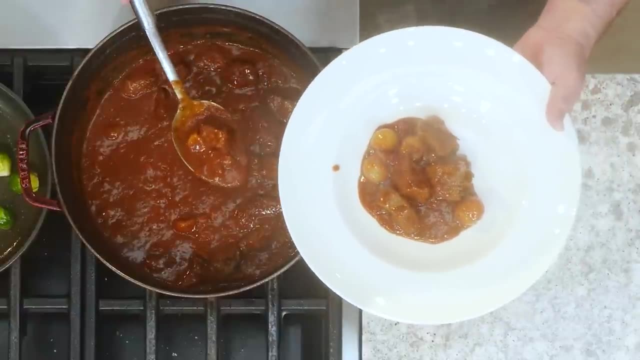 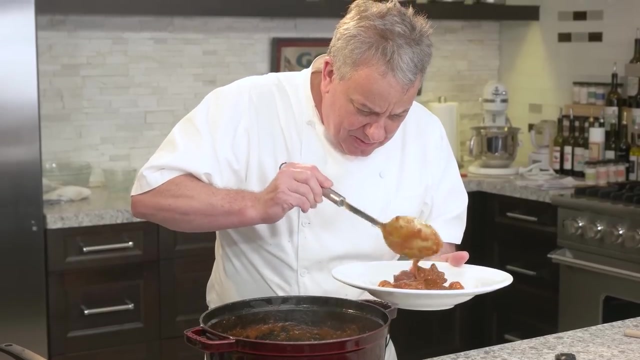 I mean, we can certainly use the mashed potatoes and we can do all that. But I got those cool little vegetables that I did- You know, I did some baby Brussels sprouts and carrots, And so I'm going to do this right there, right. 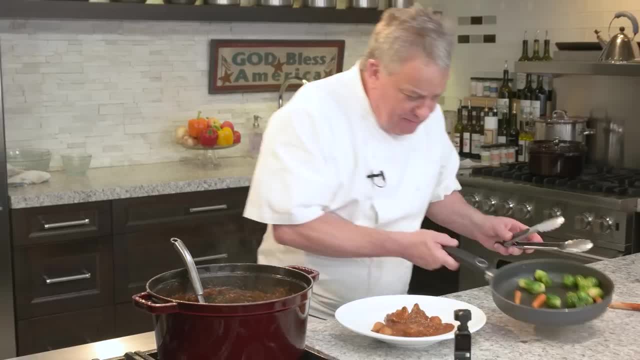 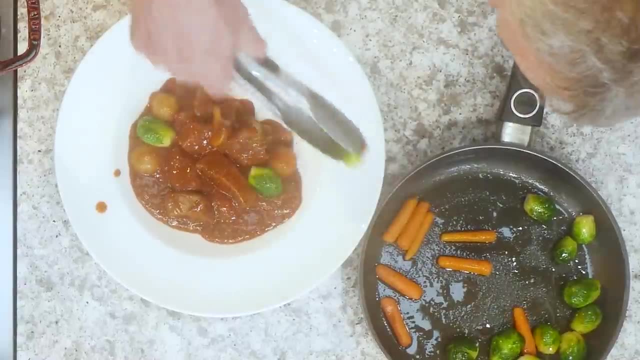 And I got. I sautéed some baby carrots and the Brussels sprouts And I sautéed them at the last minute. They cooked right, So we poached them already, Lay it down, And I just finished sautéing them in butter, real quick, you see. 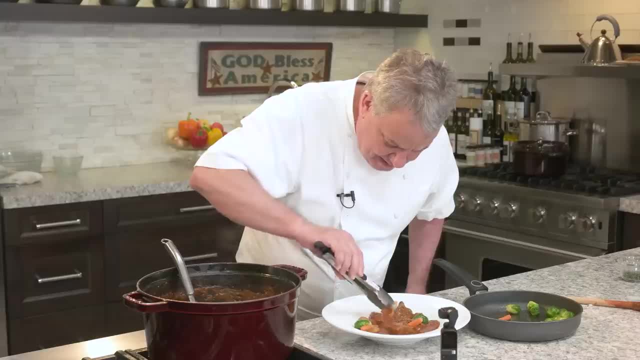 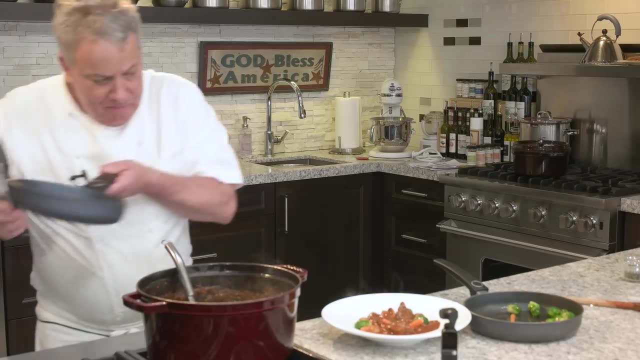 Just like that. Just really, really simple. Just let it not go crazy here. right. Just like that, right. And we got a couple of carrots in there, Nice, right. And then I got those baby potatoes I was telling you about. 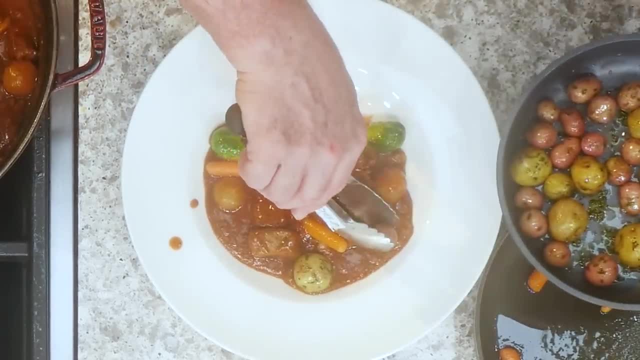 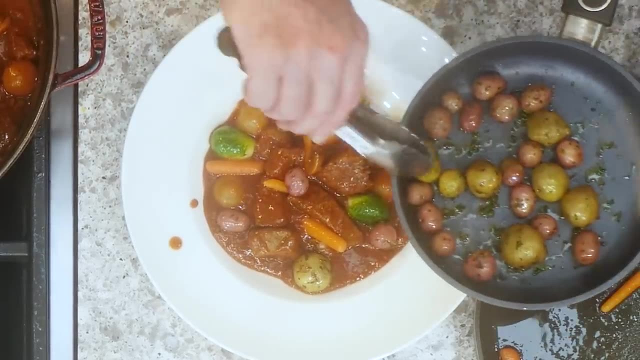 So I cooked those separately. I mean, you can cook them inside if you want. But you know what I find? I find that if you cook them inside they lose their colors and everything And they're not that attractive anymore. But they're delicious.